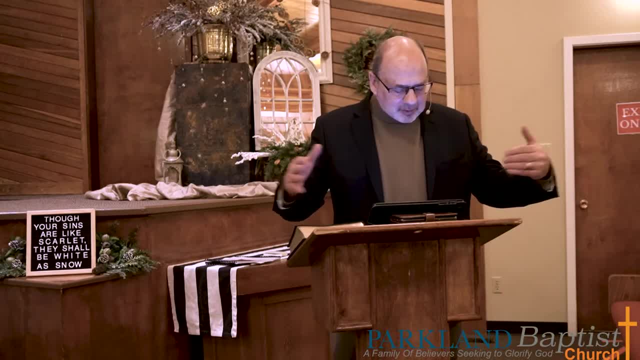 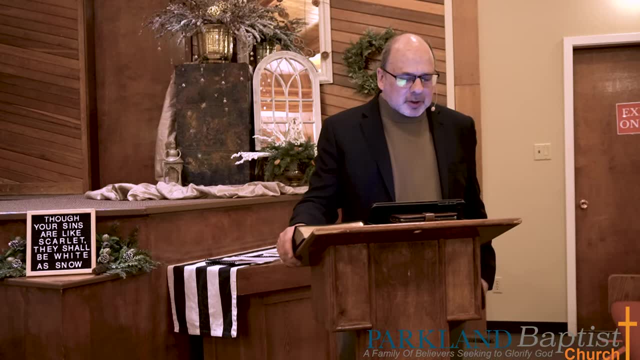 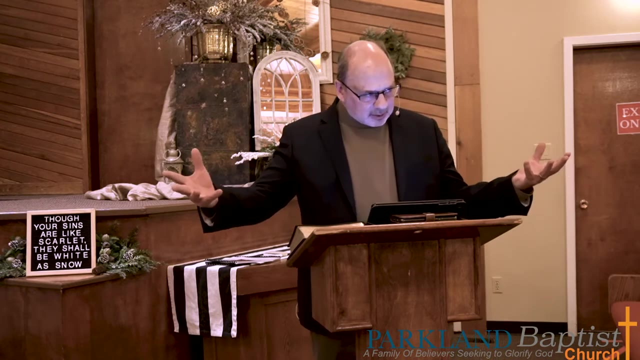 and then you know, there's a whole bunch of intermediates, but there's two on each side in terms of methods of interpretation. One is what we call the allegorical method of interpretation and the other one is the literal method of interpretation. Okay, so, 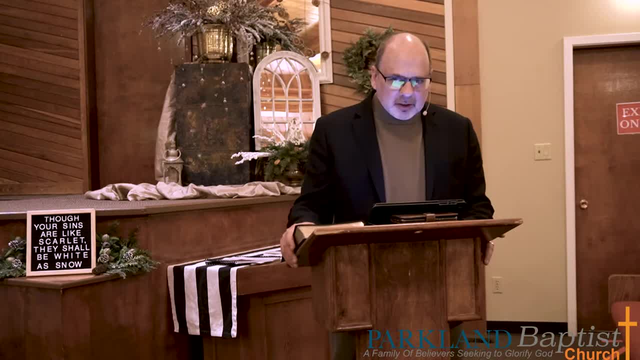 that's kind of what we're going to look at, and then we're going to land on a particular position, or at least a position that I would hold, And then that'll be the end. So that's kind of where we're going. We're going to compare. 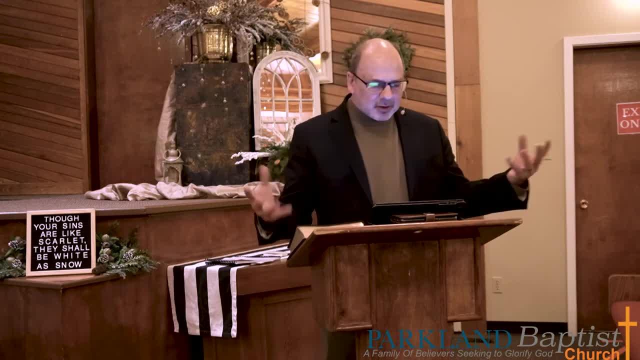 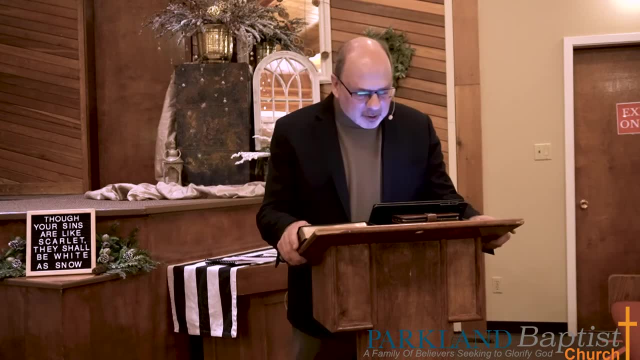 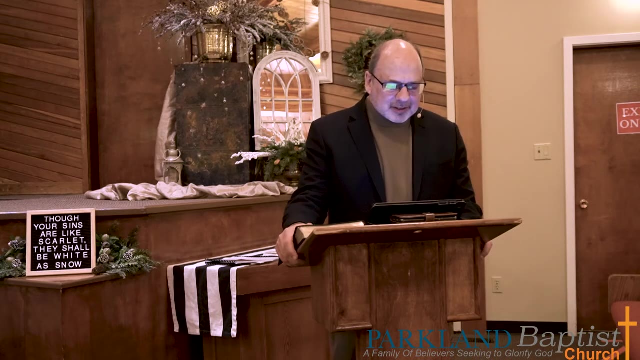 allegorical and the literal methods of interpretation to see the strengths and weaknesses of both. Let us start with the allegorical interpretation. What in the world does allegorical interpretation mean? Well, in general- again, these are all general terms. In general, it is a hermeneutical. 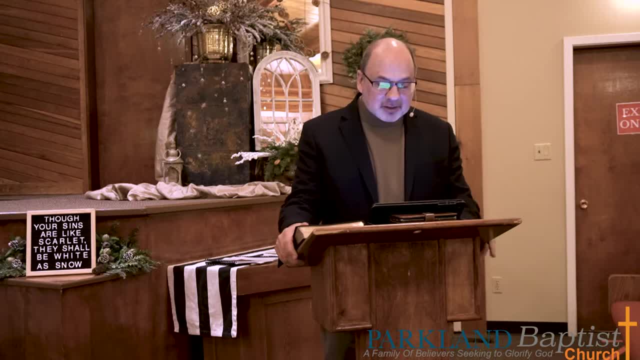 method of assigning to the literal words in the text In the text secondary meanings that are not expressly taught by the words. Okay, so this will be in your manual. if you have your manual with you, I'm not sure what page we're at. 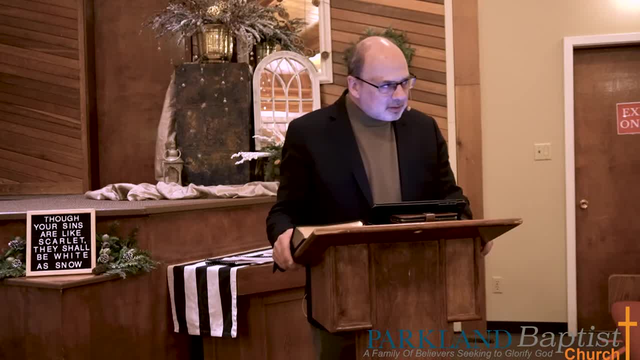 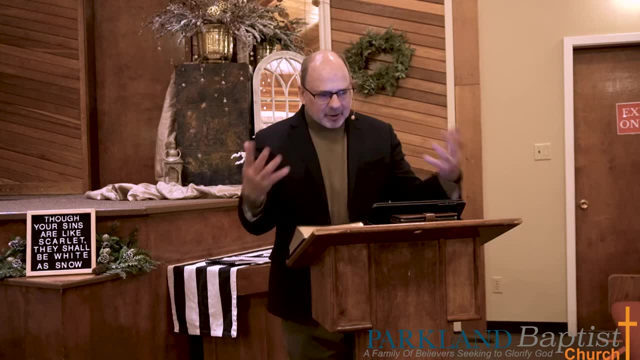 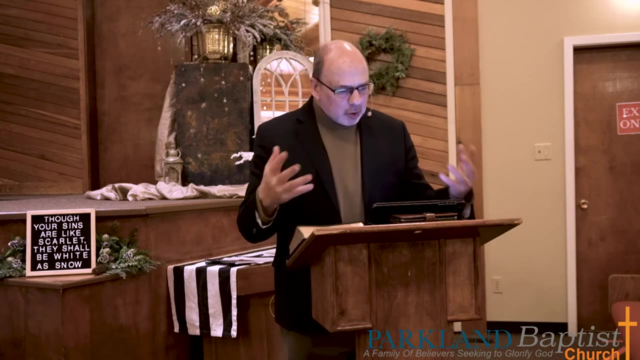 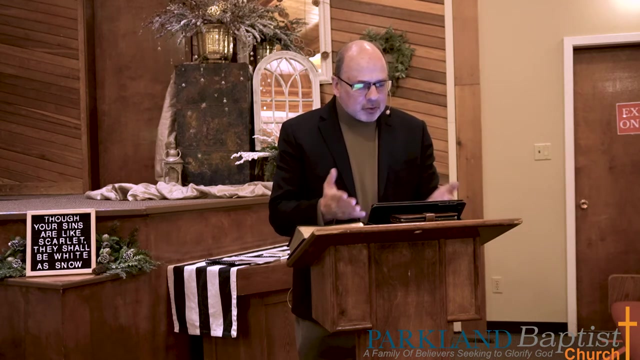 but somewhere in there, Which page 25.. Okay, so we're assigning to the literal words secondary meanings that are not expressly taught by the words. So new meanings or deeper meanings are attached to the text, Attached to the biblical words. That's allegorical. So rather than drawing out the intended meaning, 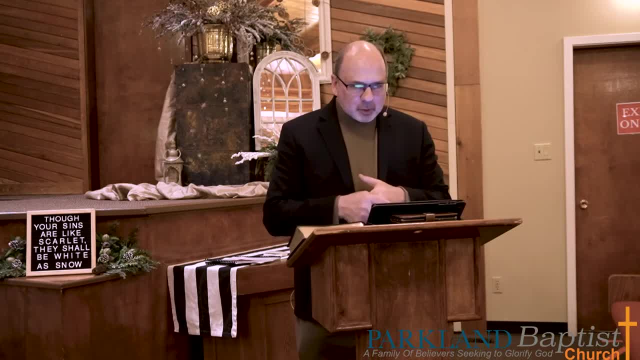 of the words of Scripture by a process we call exegesis. Ex means to draw out. Exegesis is drawing out. So in other words, there's meaning in there and our job is to pull meaning out. That's exegesis. The allegorical interpretation tends to import meanings into the words of. 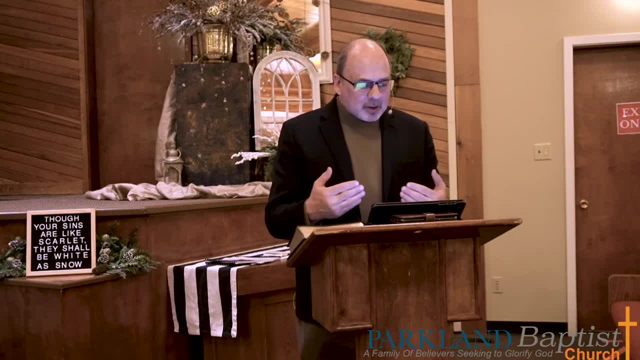 Scripture By a process that we call isogesis: Iso meaning into, Exo meaning out, of, Iso meaning into. So isogesis basically means I'm importing meanings into the text that are not explicitly there. Okay, so those who advocate an allegorical hermeneutic believe that Scriptures contain: 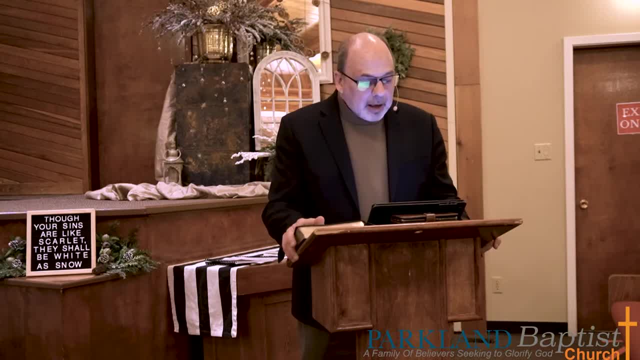 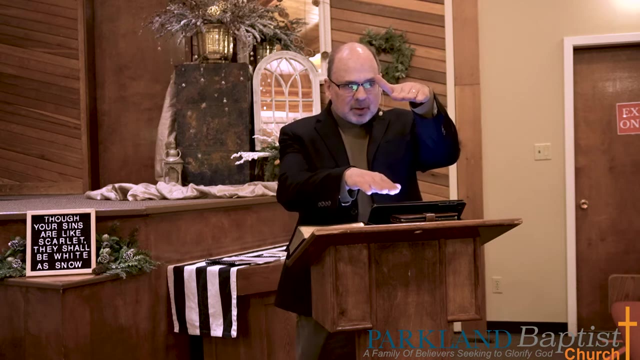 multiple layers of meaning, And it is us, It is up to the interpreter, to discover the deeper sense of the text. Okay, so, in other words, you have multiple meanings to the passage, And the job of the Bible reader, the job of 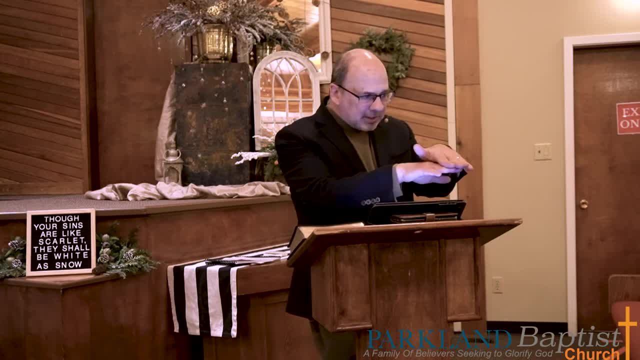 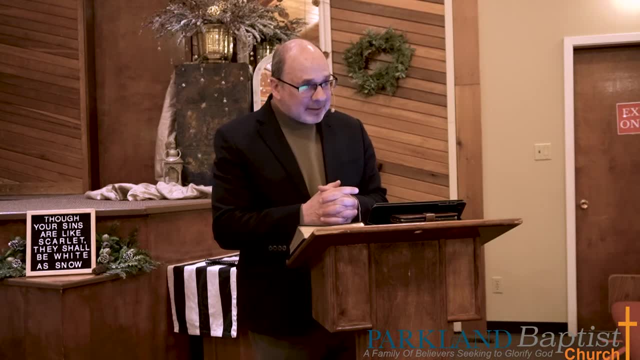 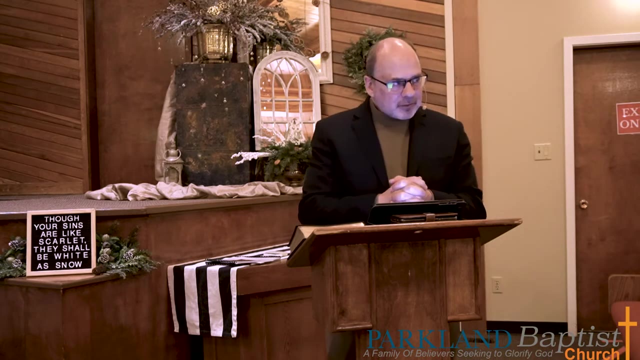 the Bible interpreter is to try to discover what those deeper meanings are. Okay, interpreters in this tradition do not deny the literal sense. They deny the literal sense of the text, But what they say is that the literal sense of the text is not sufficient. It's not the exhaustive sense of the text, There's more. 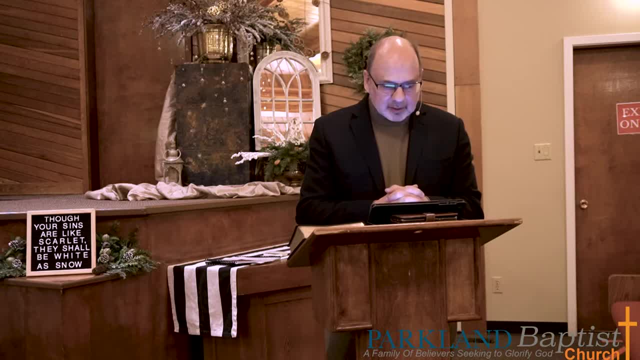 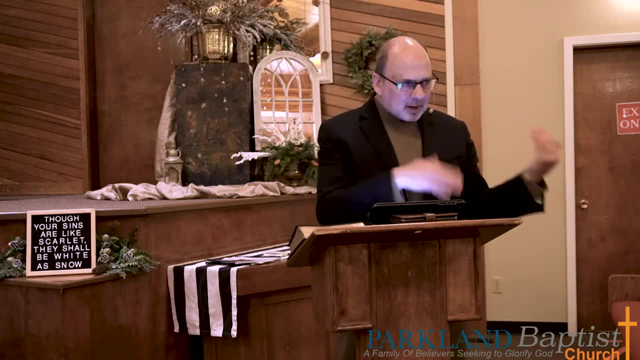 meaning, more multiple layers of meaning, And so we have to get out, get to it, And sometimes I mean some who go to the extreme would say the literal sense is not, even is not as valuable of a sense as the deeper meaning. 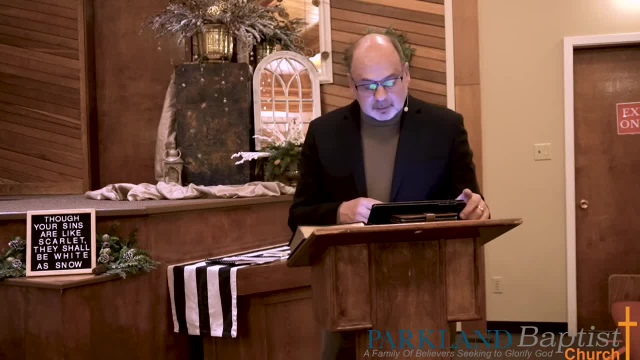 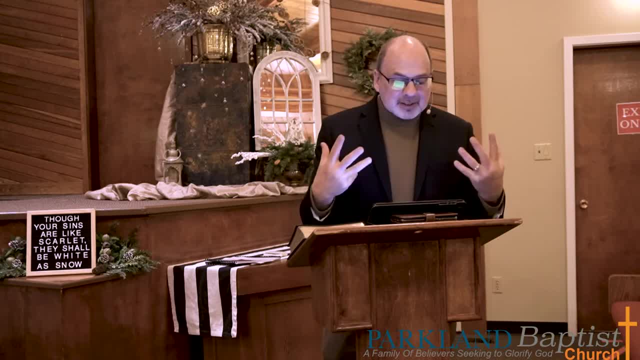 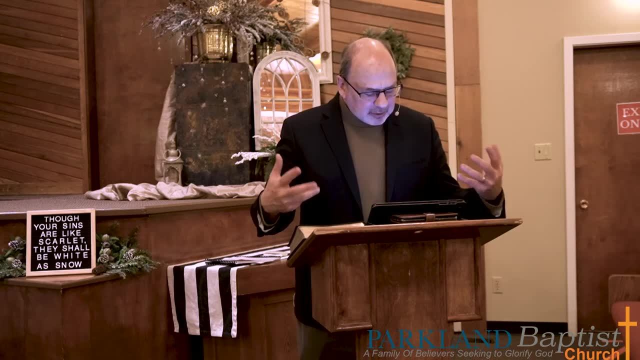 Who would express that to us, What We're going to get there? Okay, So the literal sense, particularly of historical passages, according to those who uphold or follow the allegorical method. Now I just want to say most interpreters will follow. 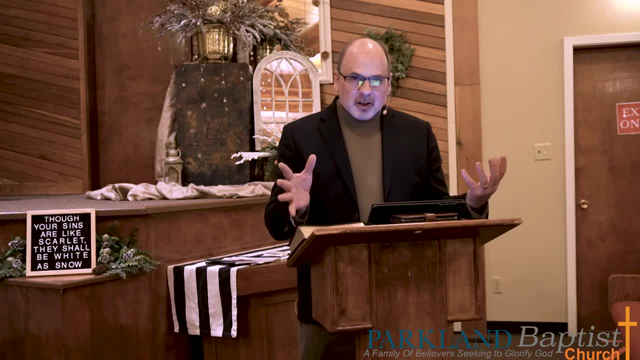 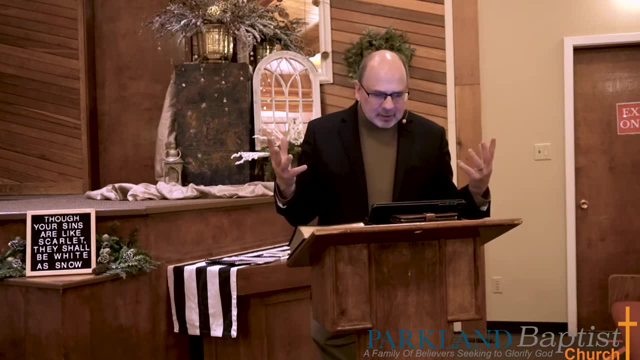 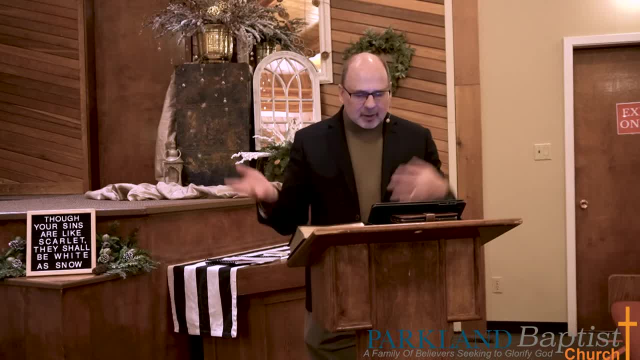 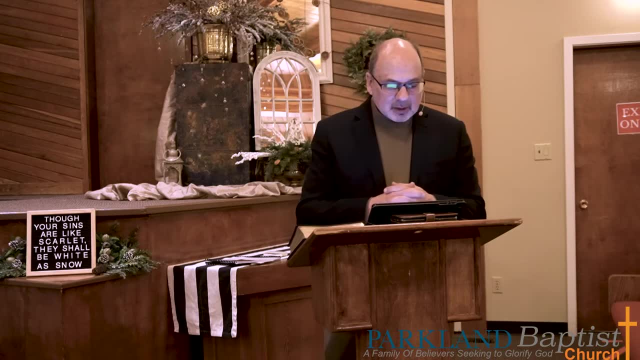 It's not sufficient. So the literal sense, particularly of the historical passages, like you know, Judges or 1 Kings or Chronicles or whatever, do not exhaust the divinely purposed meaning of such passages. The literal sense does not exhaust the divine meaning of the passage, but they also include: 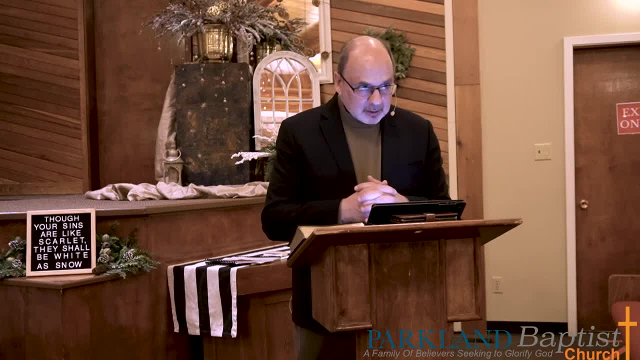 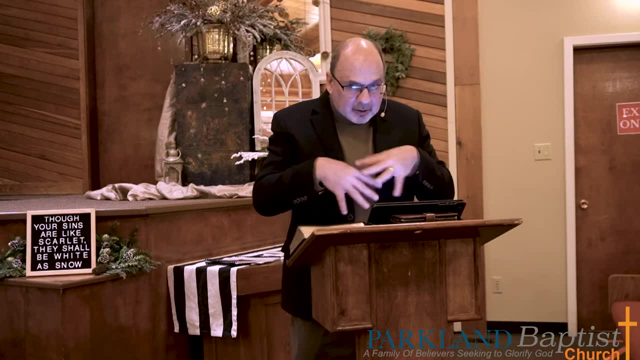 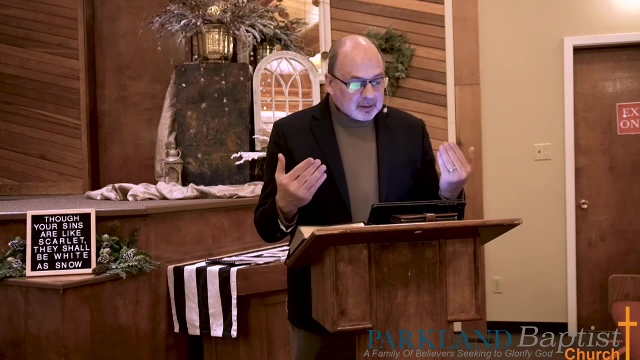 a deeper, higher spiritual and mystical sense. Okay, So that's the goal of allegorical is to find the mystical meaning, the deeper, higher spiritual meaning of the passage of Scripture. Okay, So, in every text of Scripture, in the minds of the allegorical interpreters. 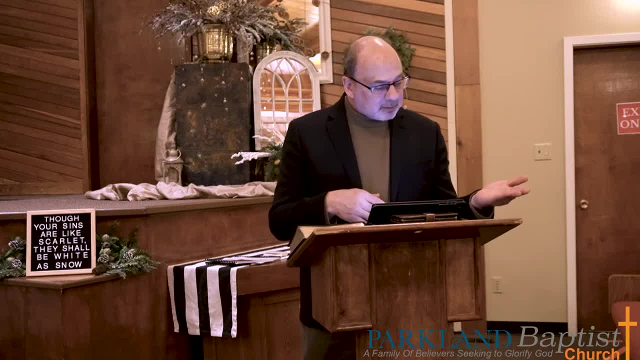 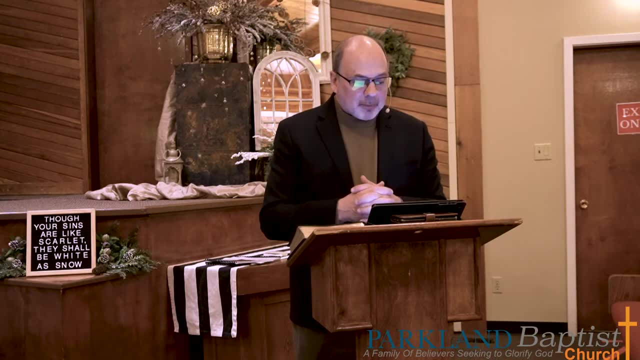 there's a two-fold sense: the immediate, literal sense, which in most cases is not deep enough, And so you've got to go to the ultimate, deeper sense. Okay, so that's where the allegorical people go. Now, how did this all start? 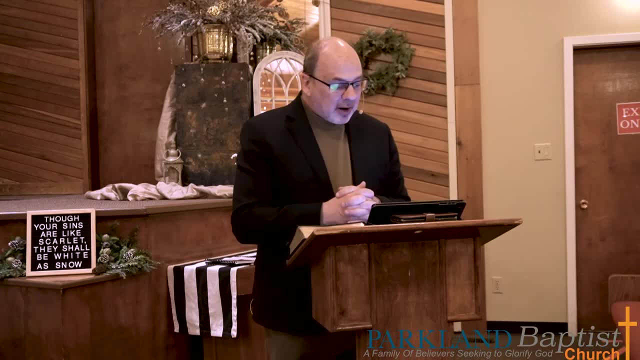 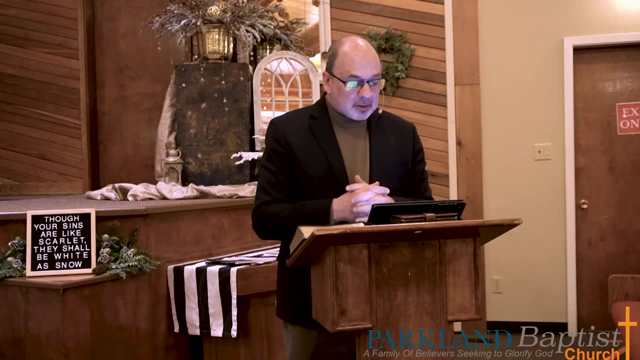 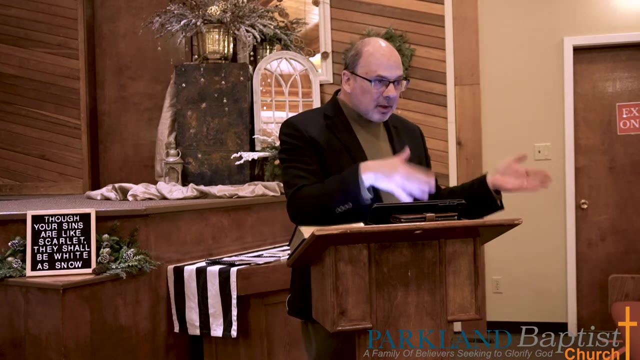 This started with some of the early church fathers, such as Origen and Clement and Augustine. Augustine popularized the allegorical method within Christendom. Here's a case in point: In the Old Testament, whenever you see the term Israel, we don't go with the literal meaning of the term Israel. 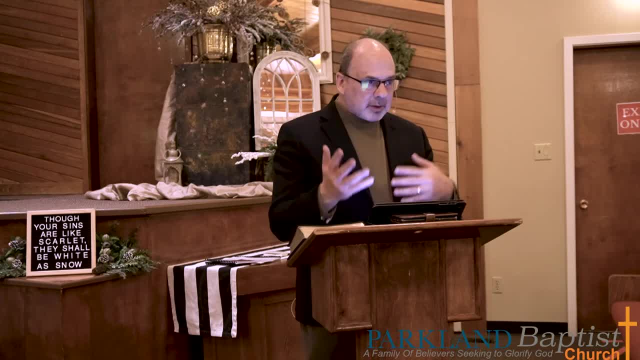 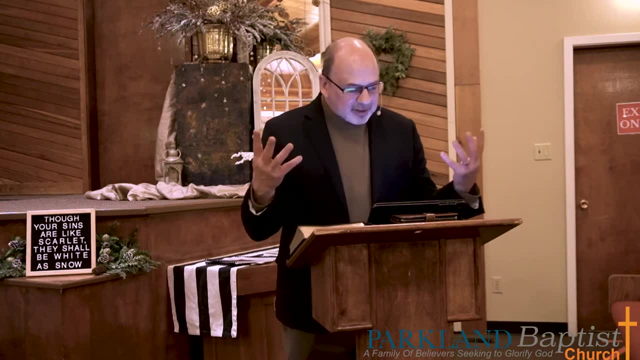 We import a newer, deeper meaning called the church. So every time you see Israel in the Old Testament according to the allegorical method, it's not literal Israel, it's now the spiritual Israel. Okay, so there's an example: Augustine and Clement and Origen did that. 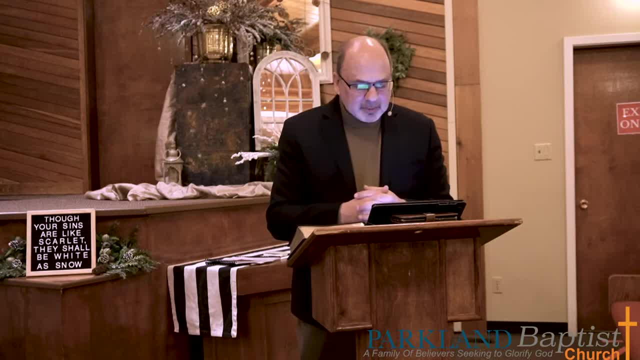 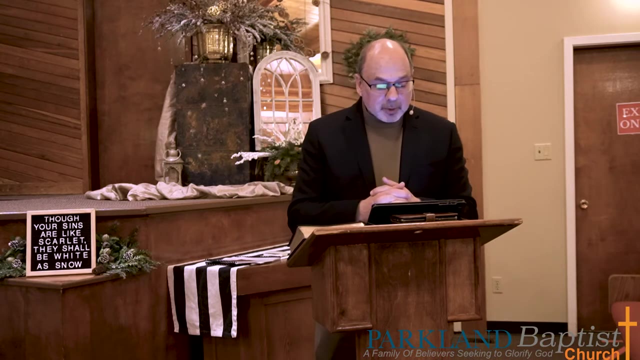 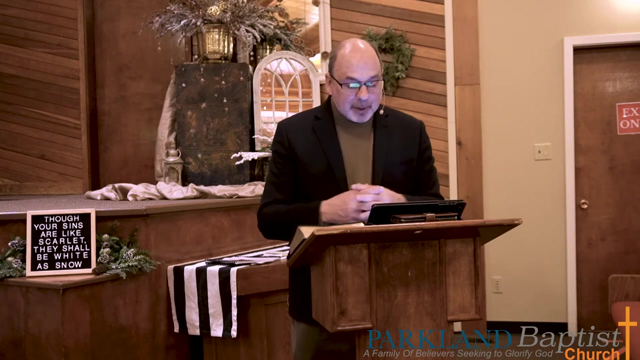 They popularized the allegorical method, And this method of interpretation- actually believe it or not- was borrowed from the Greeks of an earlier era, So it's not necessarily a historically biblical way of interpreting Scripture. It was borrowed from the Greeks And what they did is they attempted to salvage Homer from the rather embarrassing tales of the Greek gods. 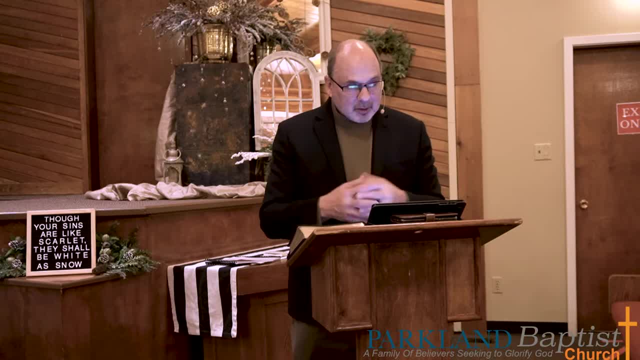 who were both immoral and capricious. So they wanted to. you know the Greeks. The Greeks wanted to soften the embarrassing tales of their gods, So they would come up with allegorical interpretations. Greeks were scandalized by the way in which Homer's gods were depicted. 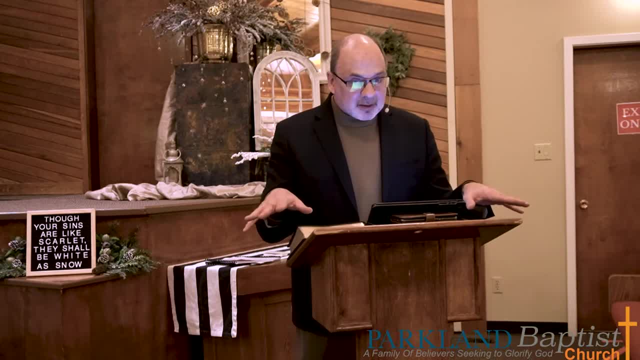 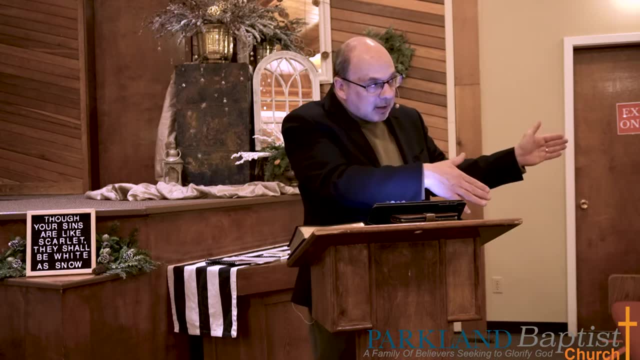 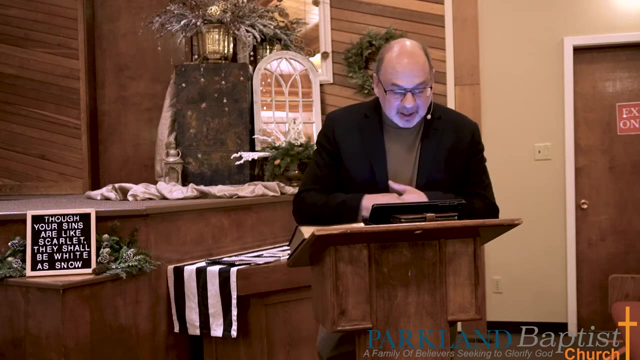 And so they sought to get past the obvious meaning of the text and offer alternative and supposedly deeper meanings that painted these gods in a better light. So that's where allegorical interpretation existed. It existed in the Greek prior to Christianity. Now. Philo was an Alexandrian Jewish philosopher. 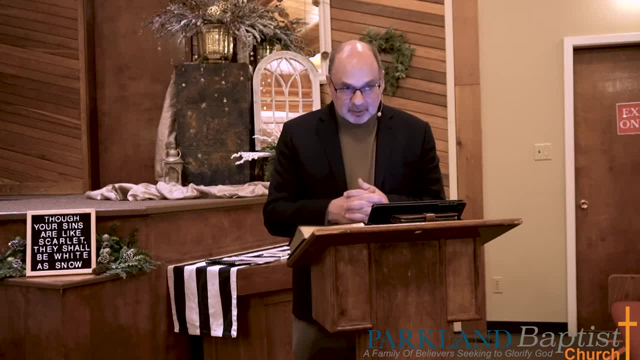 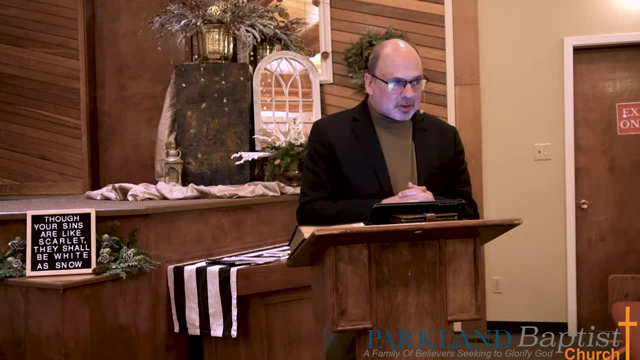 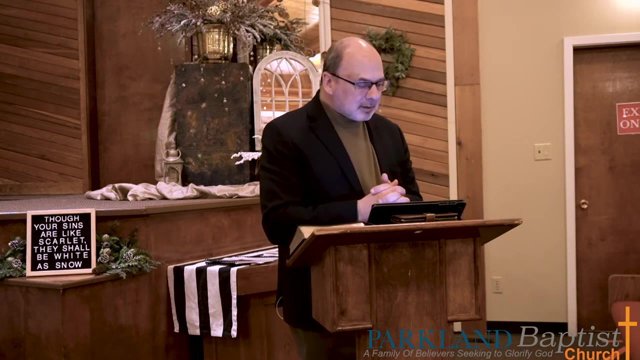 He taught that the milk of Scripture was the literal but the meat was allegorical. So if you're just going to go with the literal interpretation, you're going to remain infants on milk. So you had to go deeper. get to the meat of the passage. 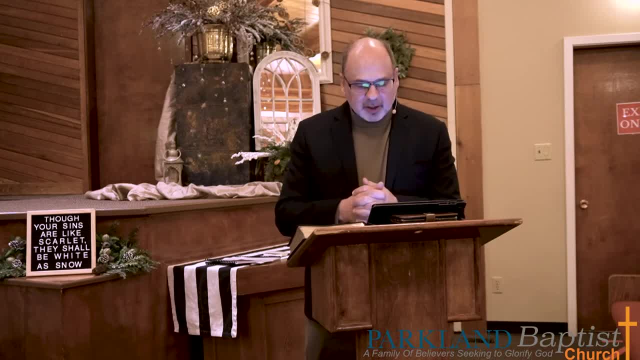 And that was the allegorical interpretation. Now Dwight Pentecost, He's no longer alive, but he was a prophet at the Dallas Theological Seminary, A very prolific writer in terms of eschatology. We may agree or disagree with his findings. 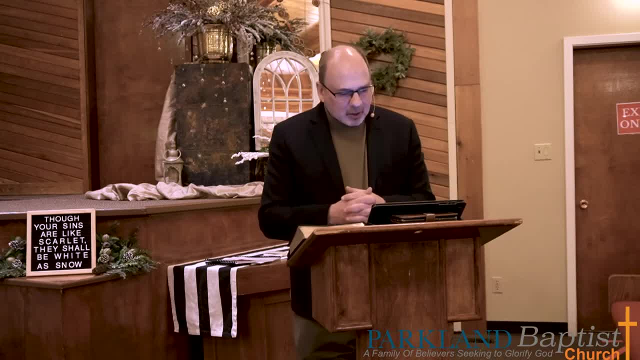 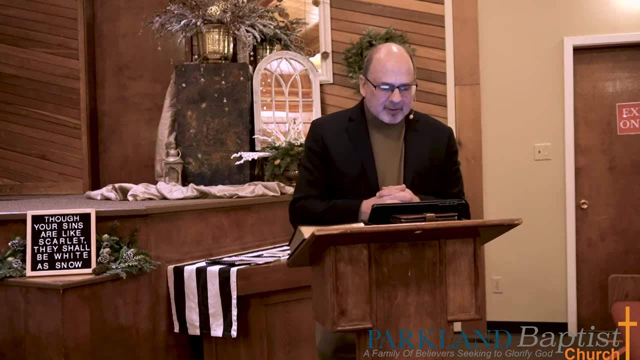 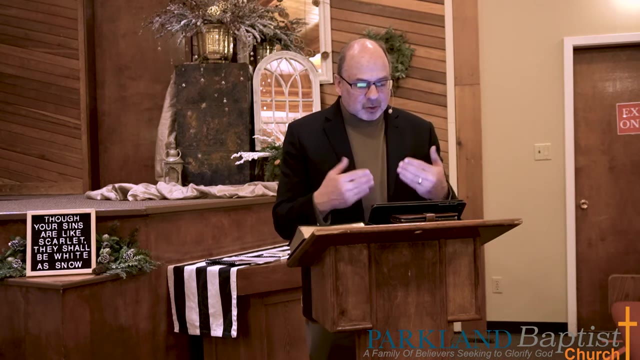 but I think what he says here concerning the allegorical method is quite insightful. He says the allegorical method was not born out of the study of Scriptures, but rather out of desire to unite Greek philosophy and the word of God. So it did not come out of desire to present the truths of the word. 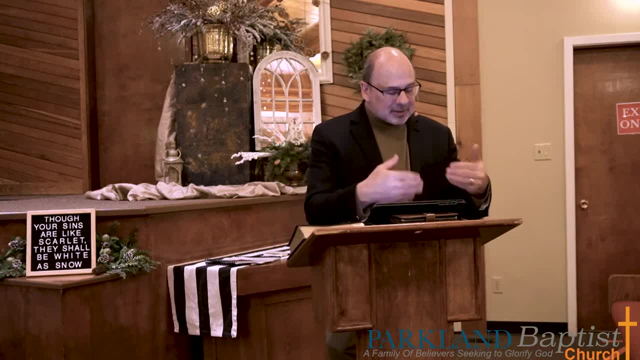 but to pervert them. So in other words, if someone uses consistently an allegorical method of interpretation, they're going to end up perverting the, distorting the words of the living God. So it was not a child of orthodoxy but heterodoxy. 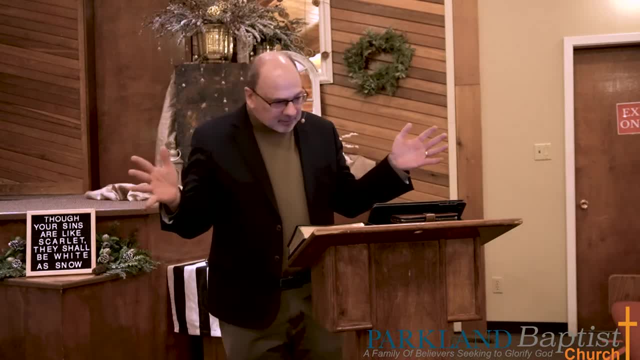 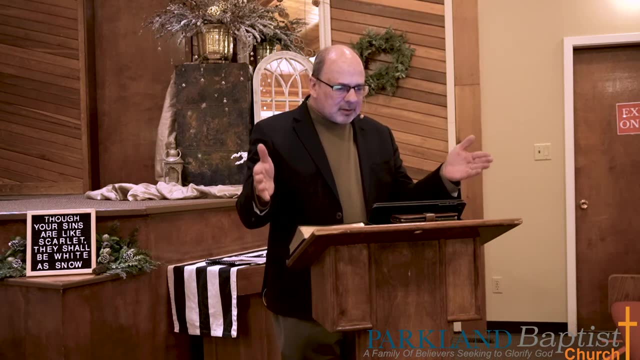 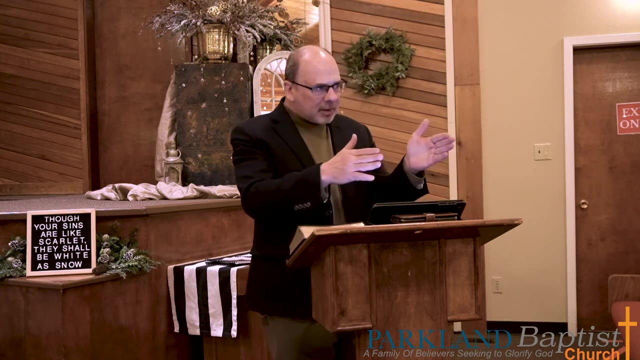 In other words, I firmly believe this. Now, you can agree or disagree with me, but if we stick to the literal interpretation of Scripture, we will not go into heresy. Heresy starts to happen when we move off of a literal interpretation. 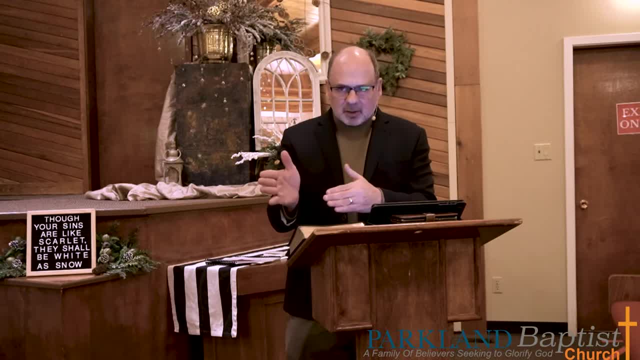 and start to go into a spiritualized interpretation or an allegorical interpretation. So orthodoxy is not the fruit of allegorical interpretation. Orthodoxy is the fruit of a literal interpretation of Scripture. So here's an example. I tend to use this: 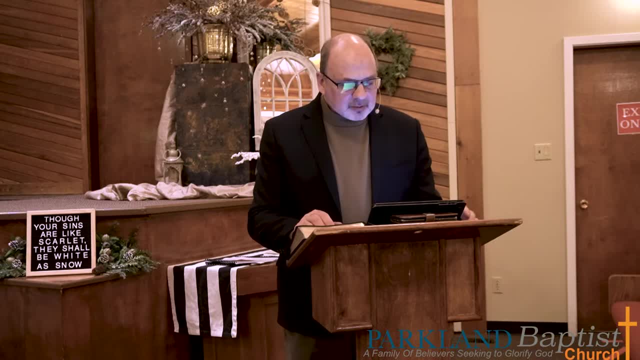 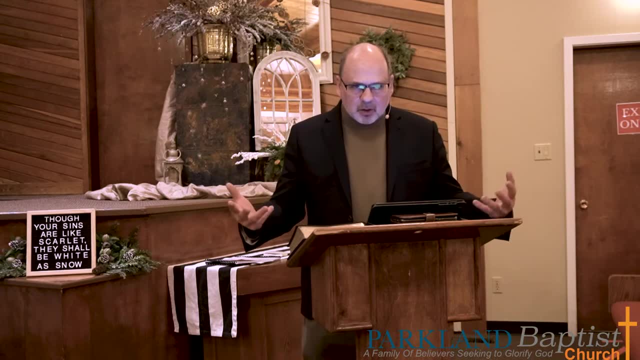 I tend to use this example because it's kind of my background. I guess, as a former science student, A contemporary example of maybe allegorical or spiritualizing the text would be uniting the modern thinking of evolution or the theory of evolution with Scriptures. 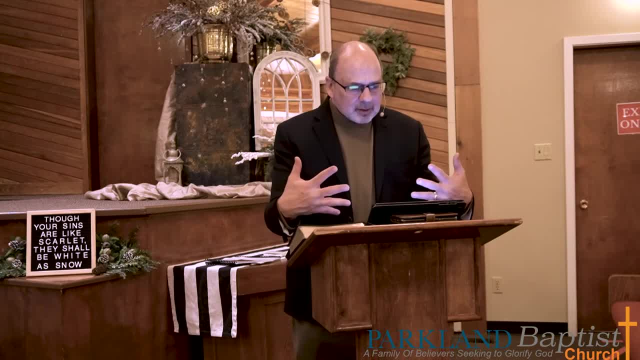 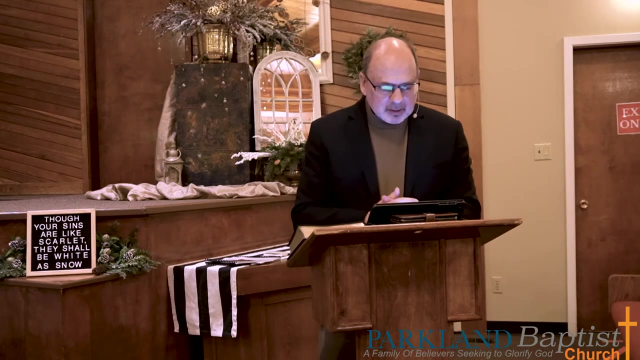 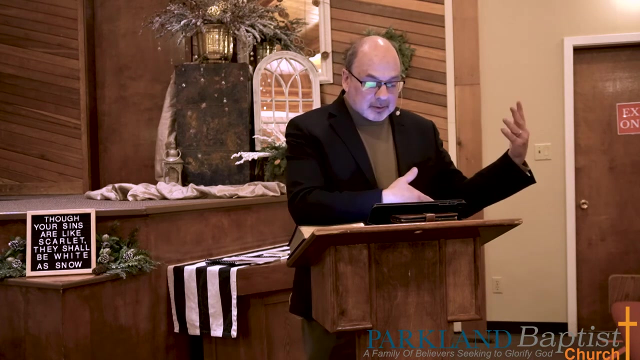 When the two are blended, we get this thinking called theistic evolution, And so this, obviously this theory is quite accepted among most evangelicals. So the theistic evolution generally accept the findings of science, but it clashes with Scripture. And so, in order to harmonize the science of evolution with Scripture, 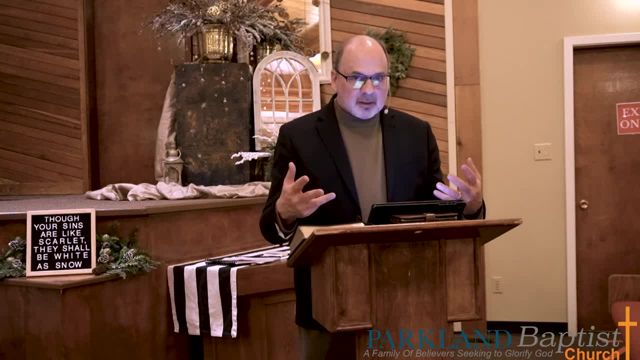 you have to start spiritualizing the text And so the text is a direct representation of the text. So you start seeing the text in the text And you start saying days in the Genesis account are not literal days, They are now long ages or long periods. 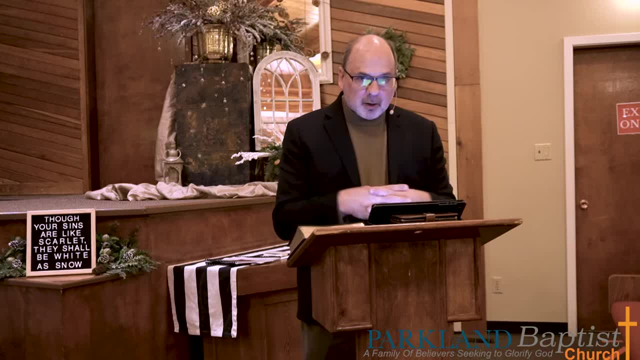 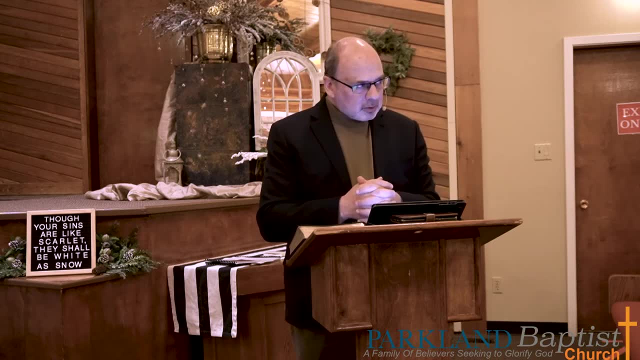 You start to go to the literal meaning is interfering with the theory and therefore we're going to chuck the literal meaning and we're going to give it a more broader meaning called theistic evolution ages. Now the thing is, if you ask any biblical scholar on the term day in Genesis 1, they would: 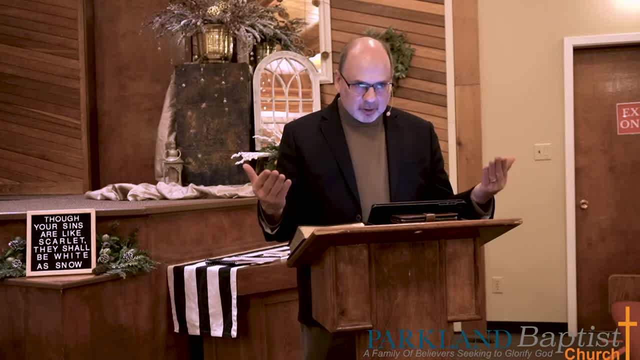 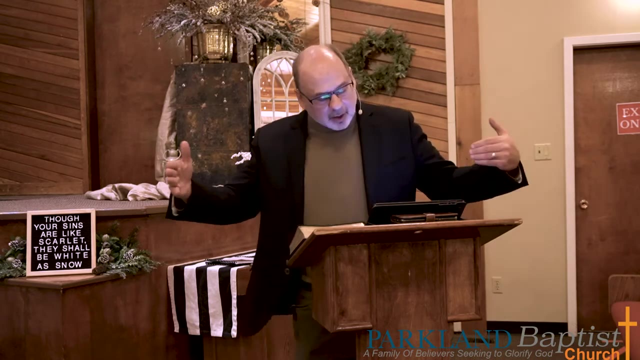 have to say that it does point to a literal day. There's very. there's no way around it Because we don't accept that or they don't accept that. then we have to come up with a different meaning to the word day so that we can now go beyond just 24 hours. So that would be an example. So 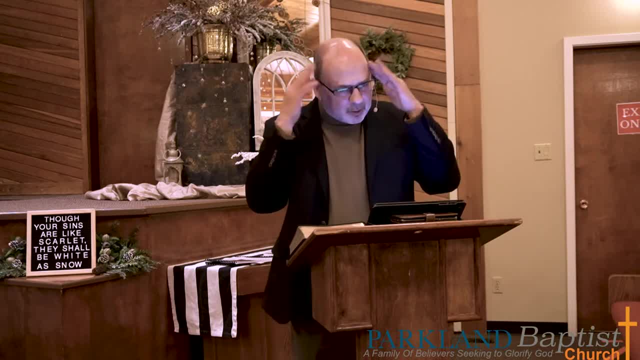 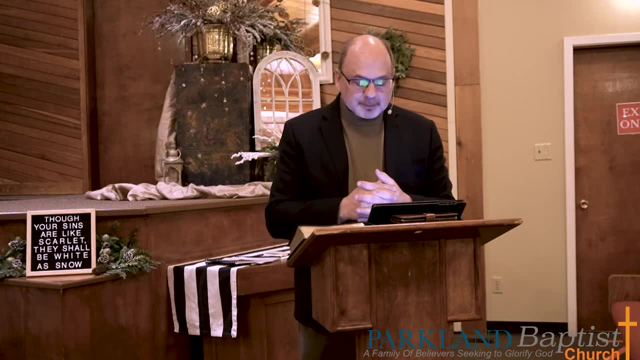 you go, you move off the literal meaning because the literal meaning doesn't quite fit our presupposition, And so we move into a more spiritual meaning of the text of Scripture. Okay, so one of the ways they do this, and we got to be careful about this. 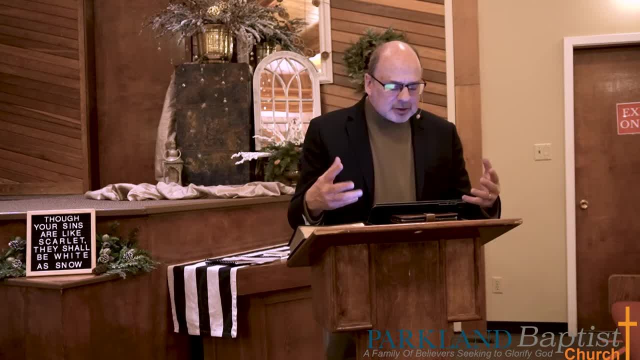 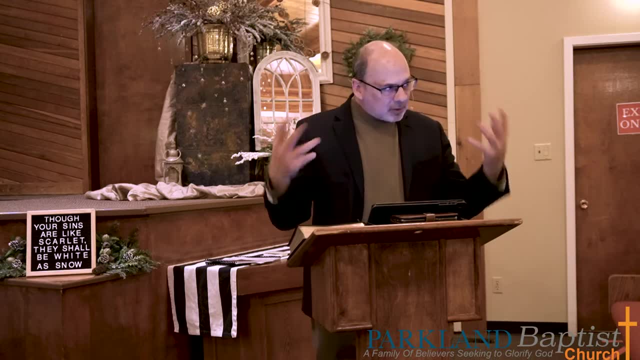 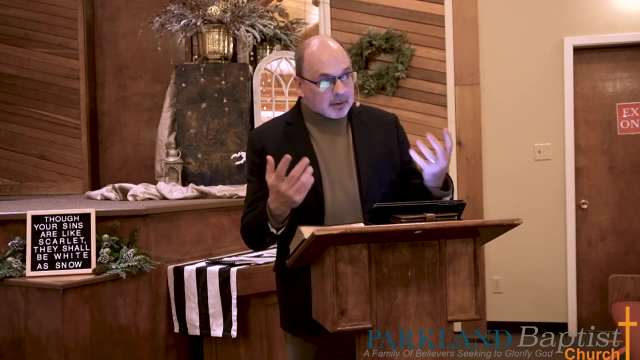 is the way that they would justify this kind of interpretation is to say: well, Genesis 1 is poetic language And therefore, since it's poetic language, we cannot take it literally. Sounds like a good justification. Okay, it's poetic language. I guess it's poetry. 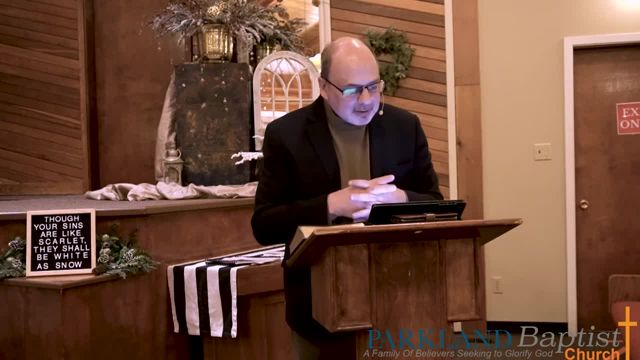 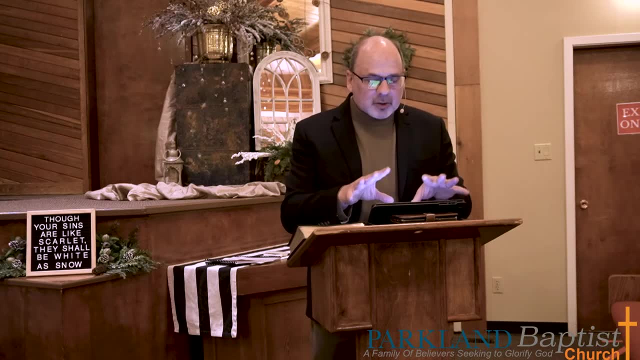 so we don't take it literally. So okay, it is long ages. Now we're going to get into different forms of speech, different genres of language. However, there were studies done on the- and I'm going off topic here, but 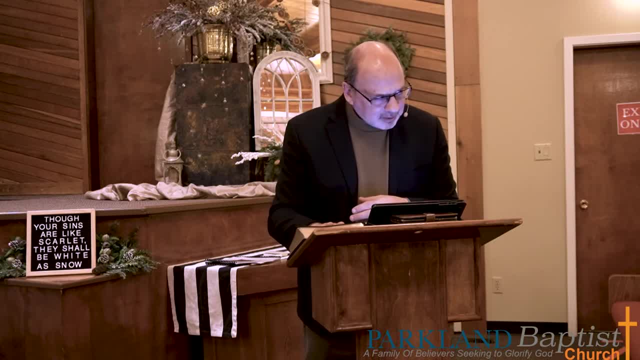 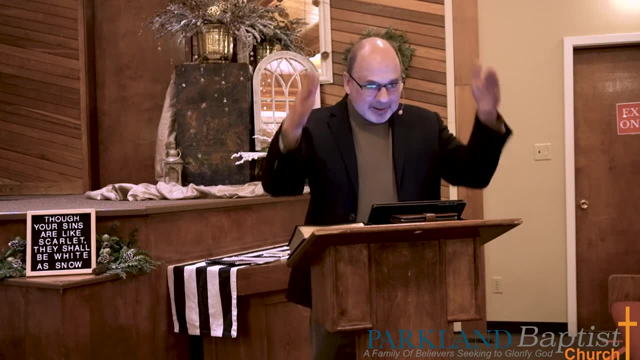 there were studies done on the grammar of Genesis 1 to Genesis 11, studying the verb forms, et cetera, et cetera. And when they studied the grammatical structure of the Hebrew language of Genesis 1, they found that the grammatical structure of the Hebrew language of Genesis 1. 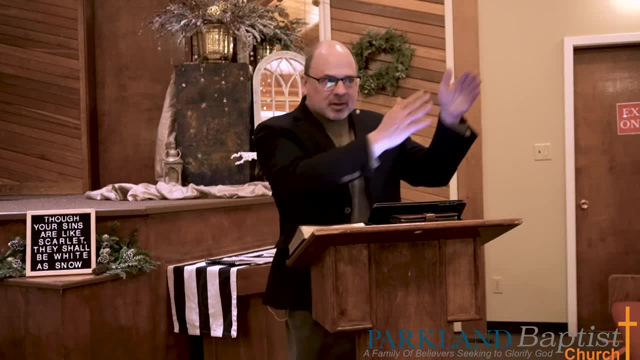 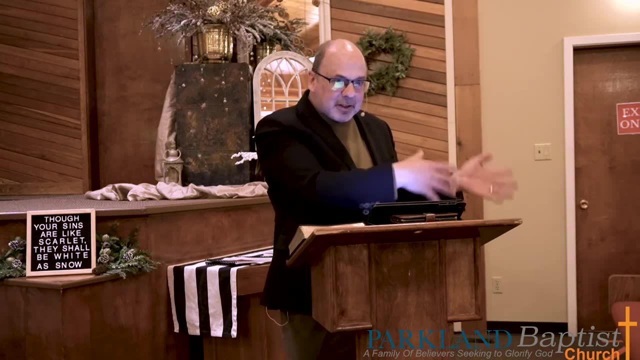 fit more with Joshua, Judges and Kings than it did with the Psalms. Psalms is poetic language. Genesis, the grammatical structure of Genesis, does not fit into the category of poetry. It fits into the category of historical narrative. 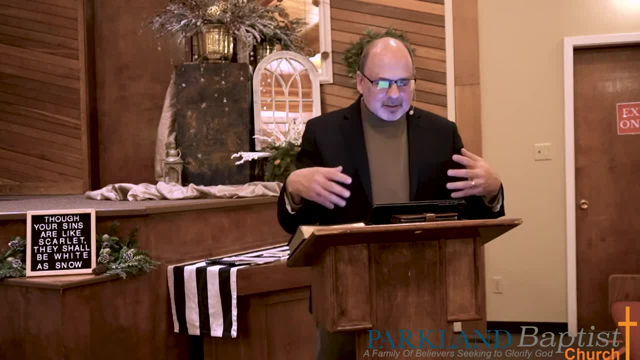 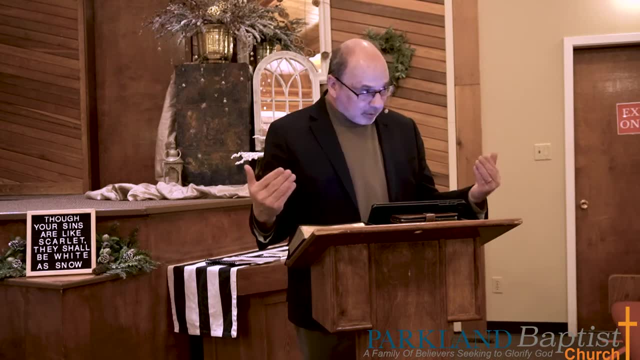 So just because someone says that it's poetic language, we have to say, well, let's verify that. We can't just call it poetic language because we want to. It has to be poetic language because it falls in the category of poetry. And so if we do the linguistic analysis of Genesis 1,, 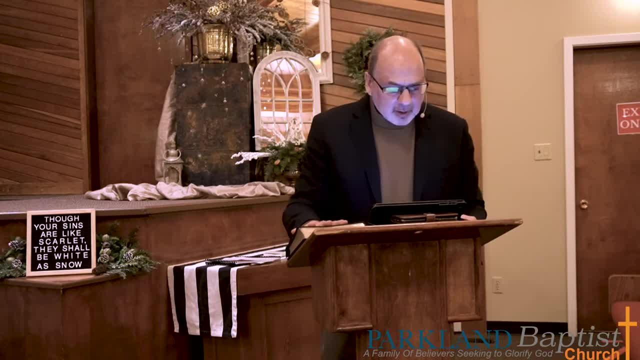 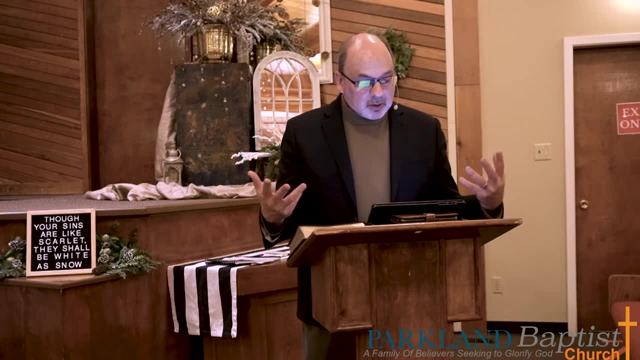 it does not fall into the category of poetry, All right. so the harmonizing process is due, via allegorical hermeneutics, going beyond the literal meaning of the text to make it say what we want it to say. So one major problem with this method: 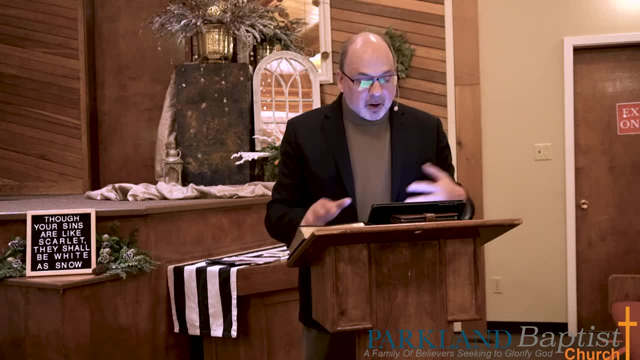 of interpreting Genesis is that if the human race evolved, well, then it messes up- and I think we talked about this before. it messes up the whole theology of sin and death. messes up what Jesus, what Paul talked about in Adam, about Adam in Romans 5, because he's talking about a historical 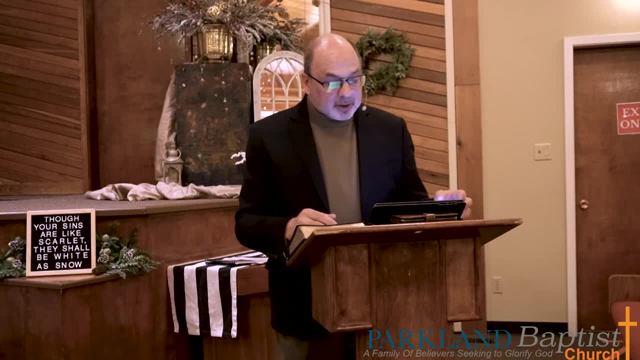 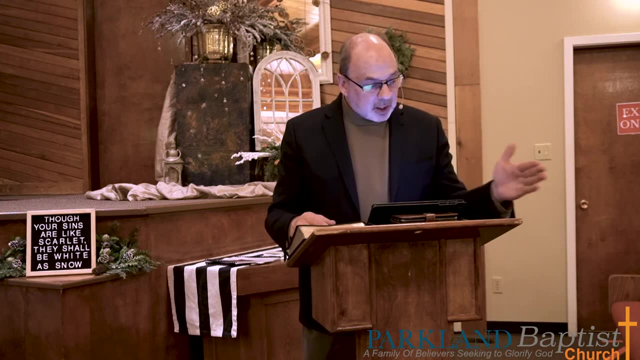 literal Adam, etc. So, then, when interpreting the scripture, regardless of the nature of the passage, a good rule of thumb doesn't matter what kind of genre it is, whether it's poetry, whether it's historical, whether it's figurative or whatever. a rule of thumb is not to import. 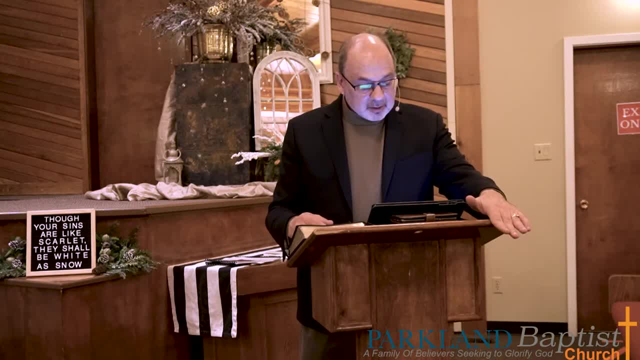 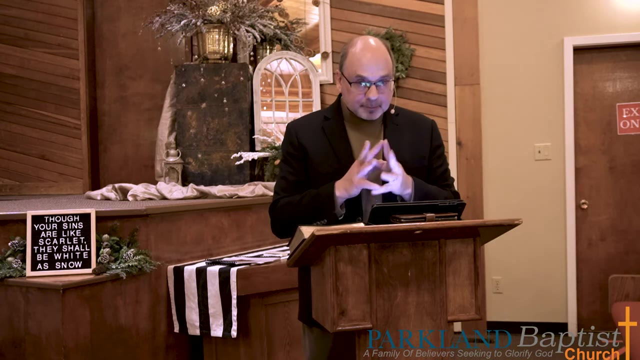 new meanings into the words of scripture. The rule of thumb is to draw out the intended meaning out of the scriptures. even if it is figurative language, even if it is poetic language, It has a literal reference point. For example, if you read some prophecy regarding the coming of Christ, the first coming of 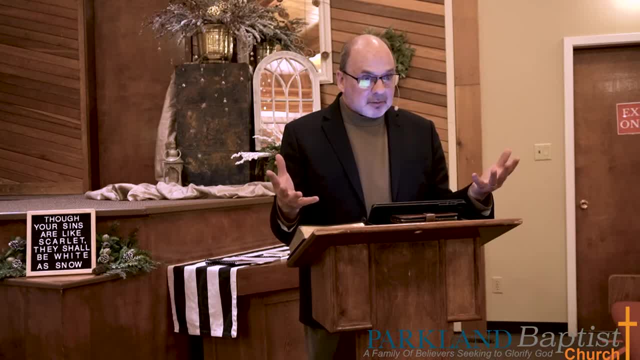 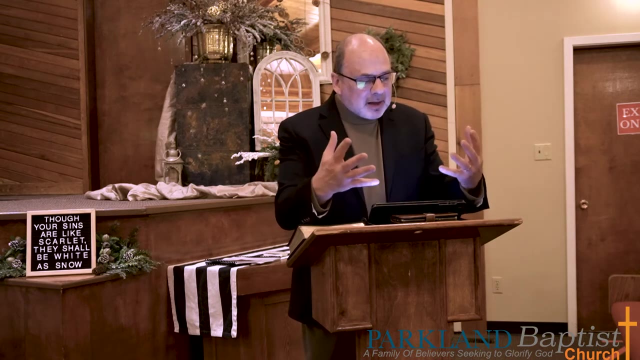 Christ. some of that prophecy is figurative language, a lamb of God. Well, is he a lamb? No, he isn't. He's a human being. but with the figurative language he acts in some ways like a lamb. So just because there is figurative language does not give us license to spiritualize. 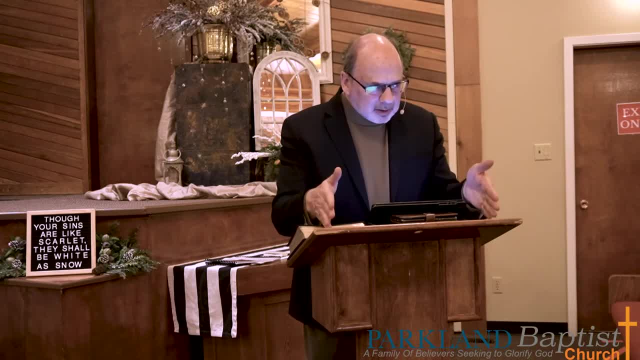 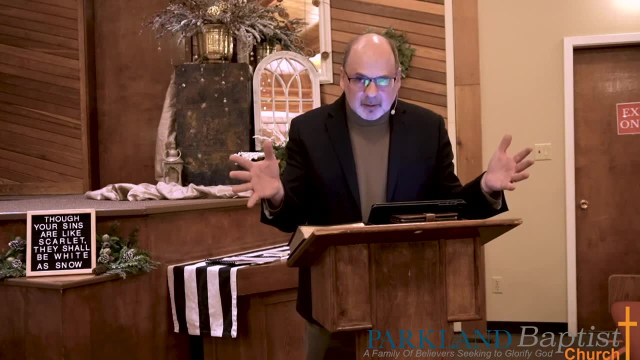 the meaning, Even though it's symbolic. language like in Revelation. sometimes you hear: well, Revelation is so symbolic we can't really figure out what the literal meaning is, Just because it's symbolic, just because it's poetic, just because it's symbolic, just because it's. 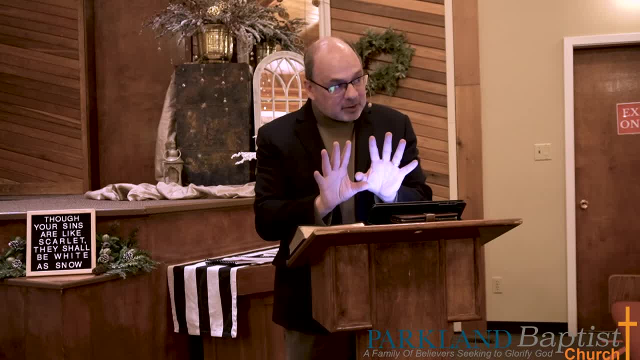 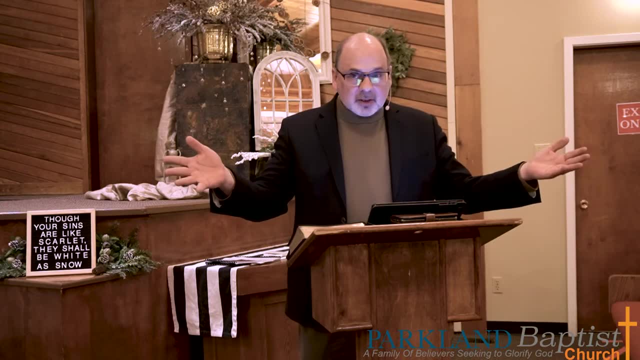 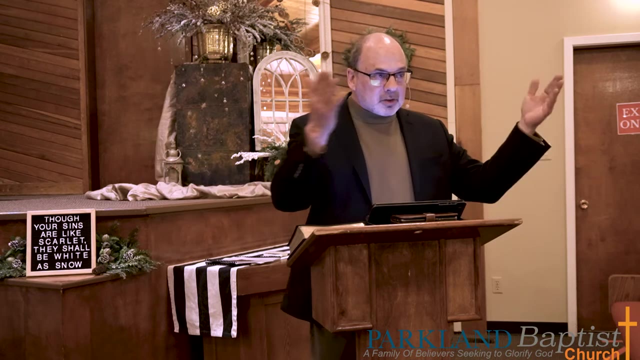 poetic just because it's figurative does not mean there is no literal reference point to the passage of scripture. Like I say, all the prophecies of Jesus. a lot of them are figurative, symbolic, but there's a literal fulfillment of those figurative passages. 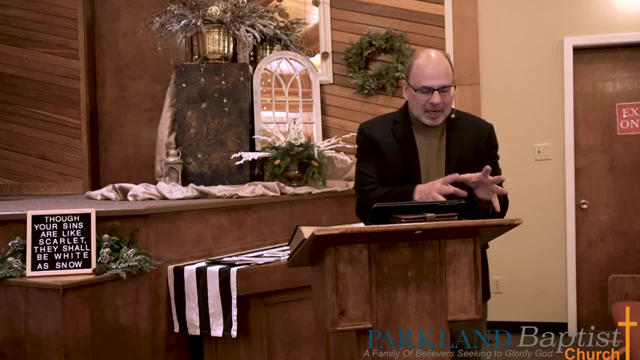 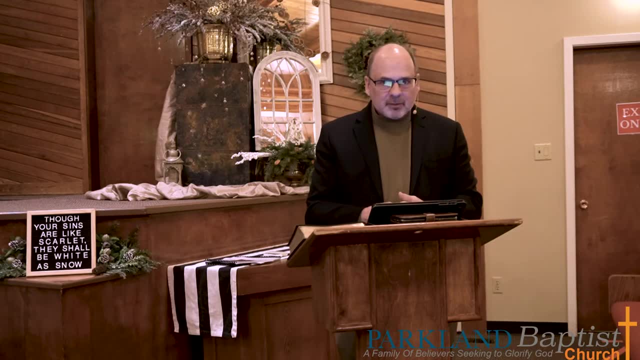 Right, Okay, So the type of literature doesn't give us the license to spiritualize the interpretation, It just tells us. well, we have to figure out what these symbolic meanings are pointing to. What literal reference point is it pointing to? For example, I remember hearing someone say: if you 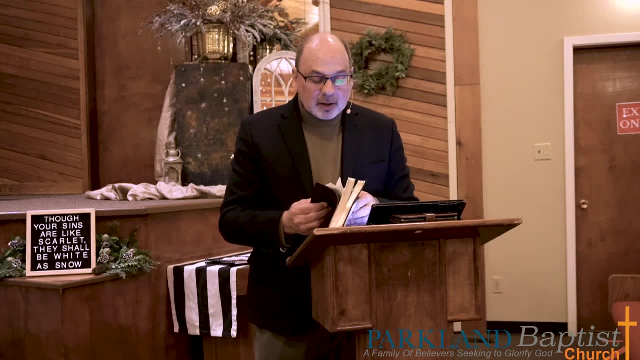 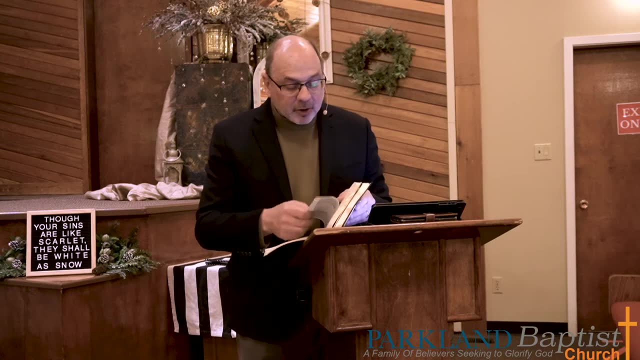 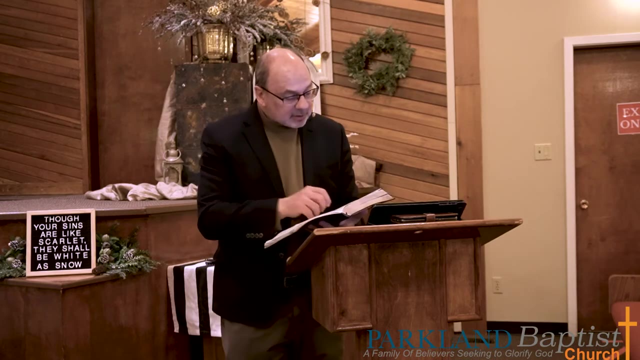 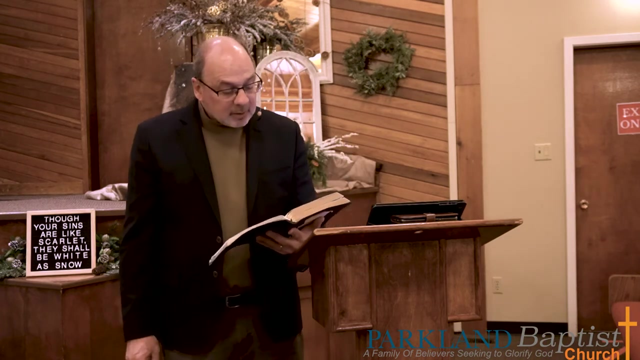 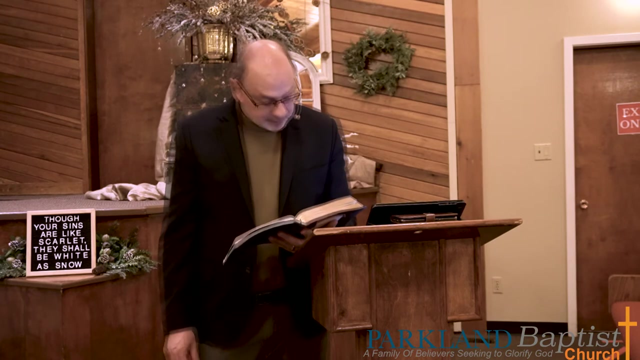 go to Galatians. you know where Galatians Paul talks about. he gives an allegory. He talks about Hagar and Sarah, referring to Hagar being the bondwoman and Sarah being the free. That was in Galatians 4, 21 to 31.. Now Paul does say somewhere in there, in verse 24 of Galatians 4, what does? 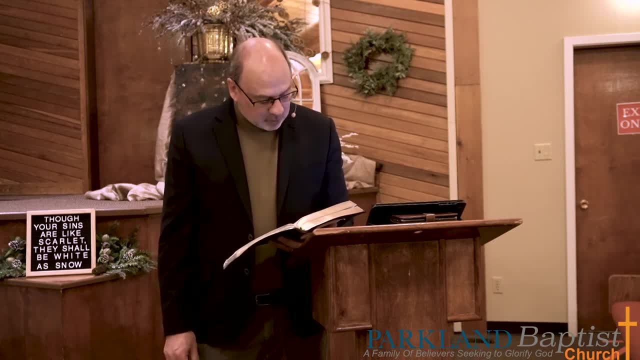 he say Genesis 4, 24.. He says this is allegorically speaking. So what he's telling us is the illustration that he's giving here is allegorical, But that doesn't mean that we interpret this allegorically. No, it still requires a literal interpretation. 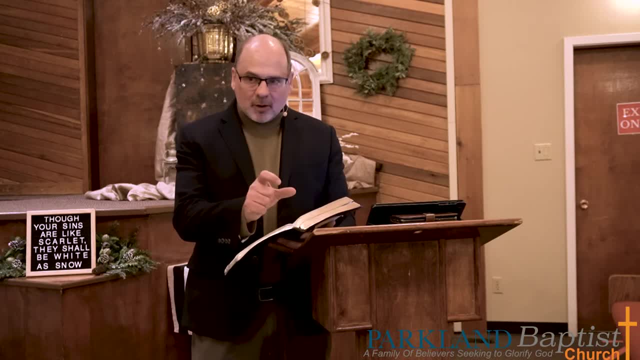 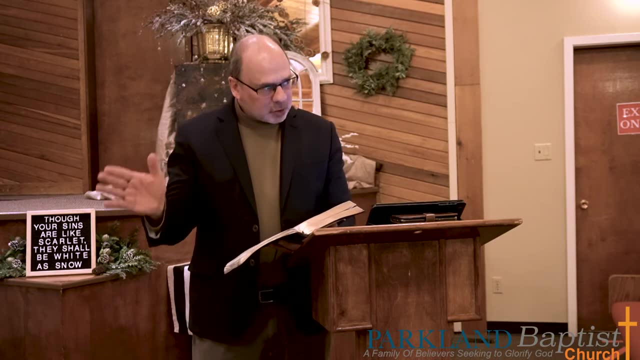 but the genre of the writing is allegorical. So we have to be careful that just because something is allegorical doesn't mean that we interpret it non-literally. Just because something is figurative doesn't mean we interpret it non-literally. That's all I'm getting at. 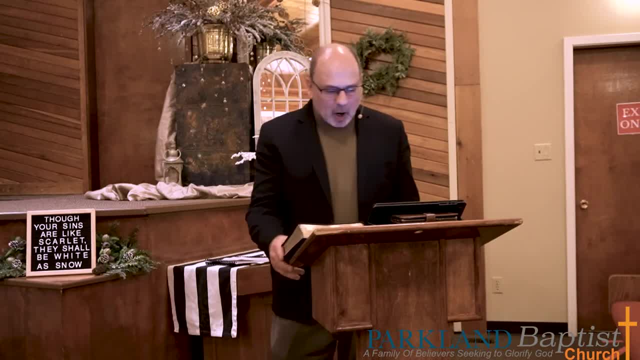 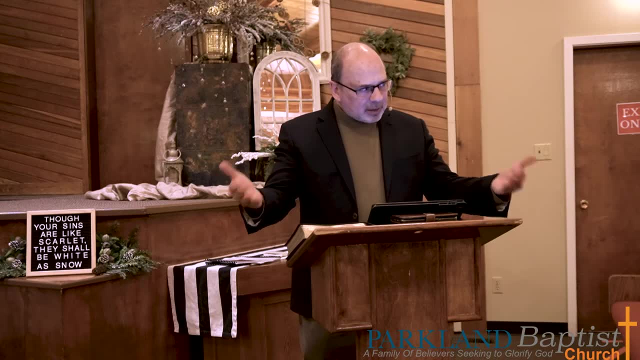 Okay, I was just reading mine, because this may be an allegory. Oh yeah, I don't have the may in there, But what Paul is saying is: I'm giving you an allegory, but he doesn't say: interpret this. 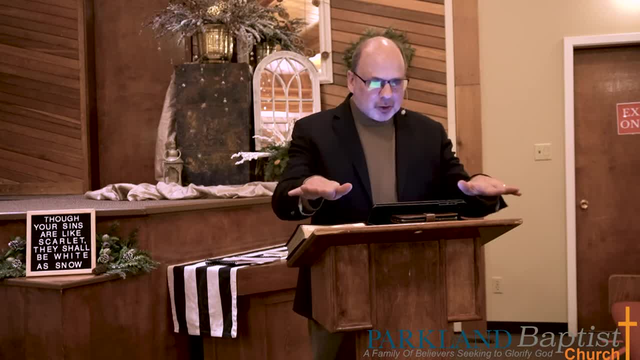 Allegorically. So the allegorical method tends to introduce new meanings to the text And in fact what happens is that if you read some of the church fathers interpretation who go allegorical, it's like all over the map. I mean there is no way to determine whether their interpretation 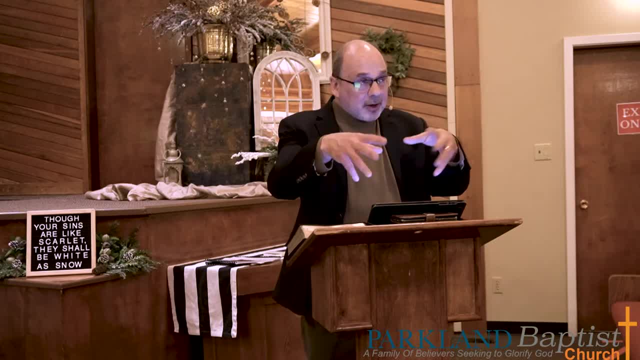 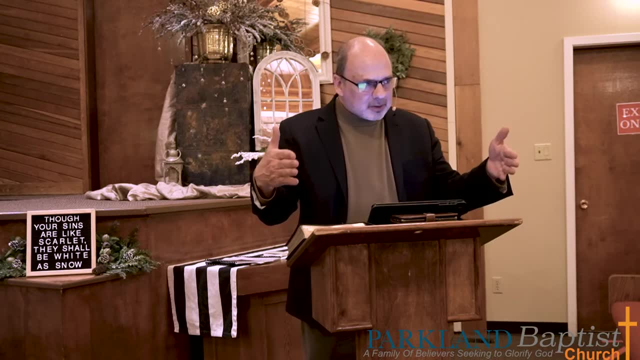 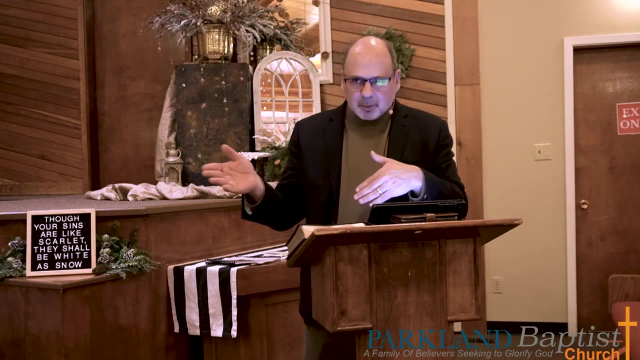 is correct or not. They are all over like this: this thing refers to this and refers to that, and- and there's nothing to drive the true meaning of this, of the text- It's one person's opinion against another, It's one person's interpretation against another. Now, if you 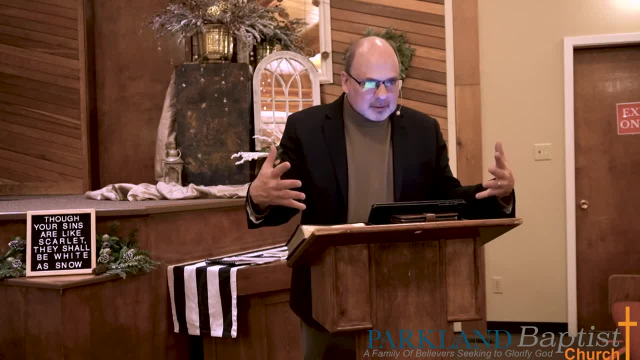 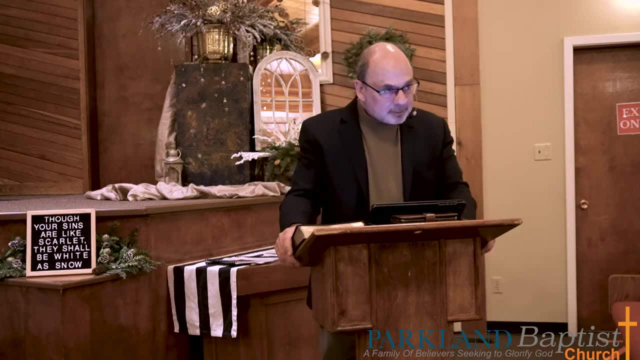 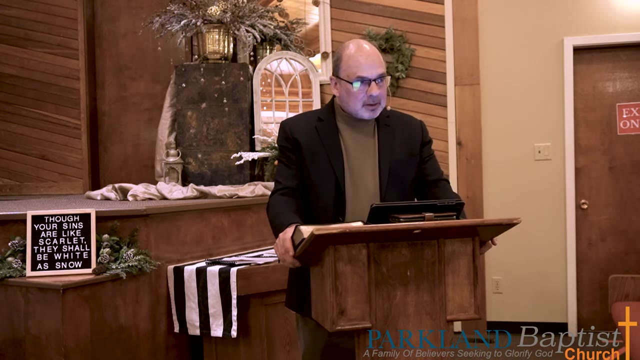 have a literal interpretation, then there's a universal understanding, If we can get at that little interpretation Basically. you're saying, just to get this straight, allegorical is figurative, Figurative interpretation. So there there is the type of text, the type of type of. 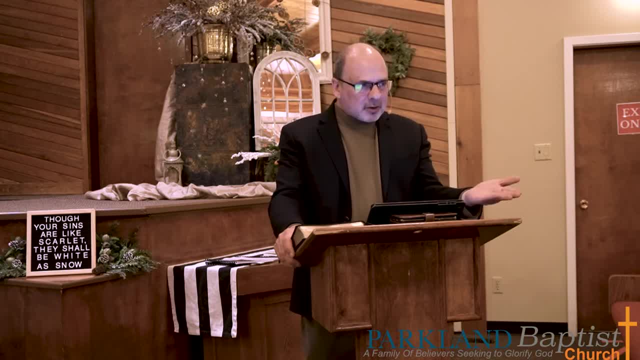 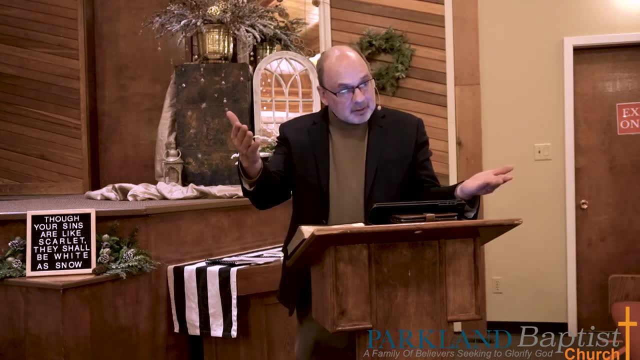 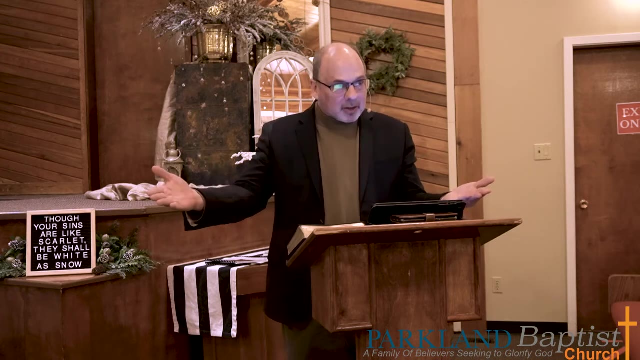 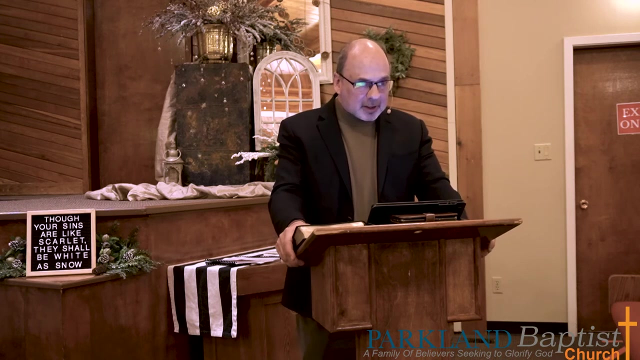 literature. there's poetic literature, there's historical literature, there's figurative literature And there's a type of understanding that literature, either understanding it literally or understanding it spiritually. So we're talking about understanding the text. So I'm appealing for a literal interpretation of scripture and not a spiritual interpretation of scripture. 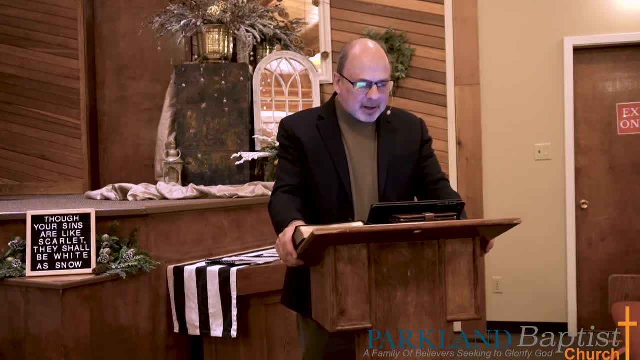 So let's look at the literal method of scripture. This method is sometimes referred to as the historical grammatical method of interpretation. What we tried to do in this process was we try to figure out what the text meant to the original audience. Okay, 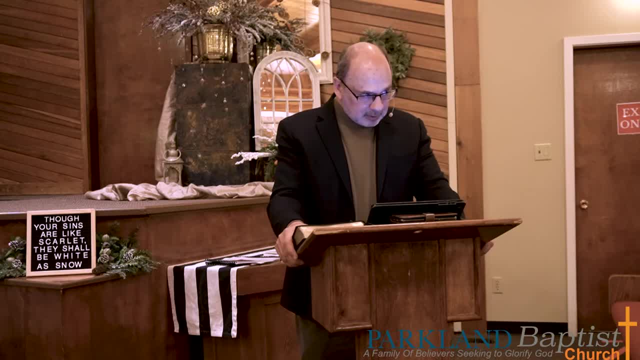 so we're trying to understand what did Isaiah mean to the original audience, or how did the original audience understand what Isaiah was saying on policy and whoever reading right? So we're trying to figure out what the text meant then to the original audience. And toрат water experienced by Isaiah2 novelism gives an explanation for why the historical 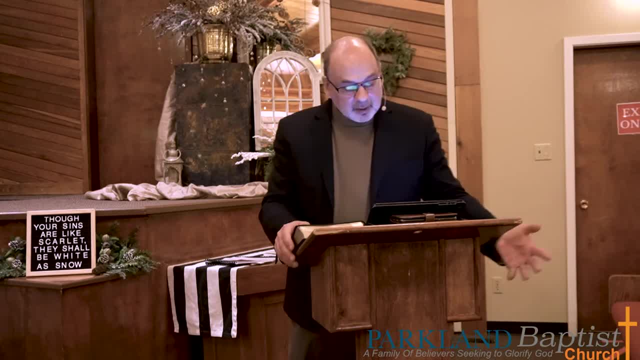 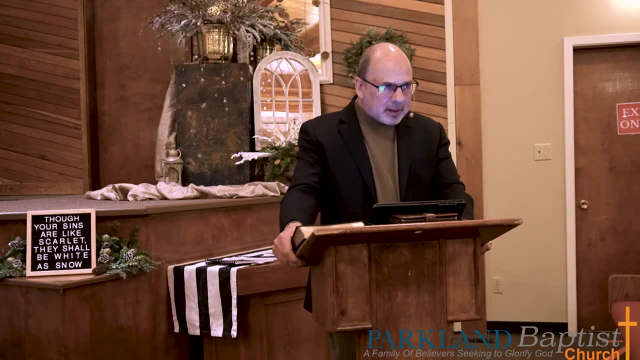 then, at the time that was written, before we move into how it applies to us today. I've always said this before and I'll continue to say this: What the text meant then is what the text means now. Meaning doesn't change, Doesn't matter how many centuries or thousands of years we've. you know the text was written. 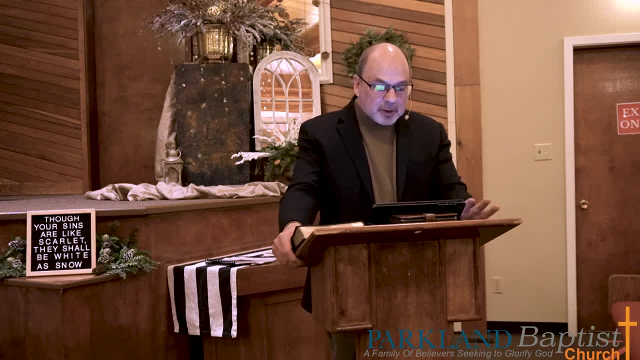 What it meant then is what it means today. Okay, so the spiritual applications are found by understanding the literal meaning of the biblical text. Okay, so we're going to reclaim the literal method of interpretation and learn a three-step process to this strategy. 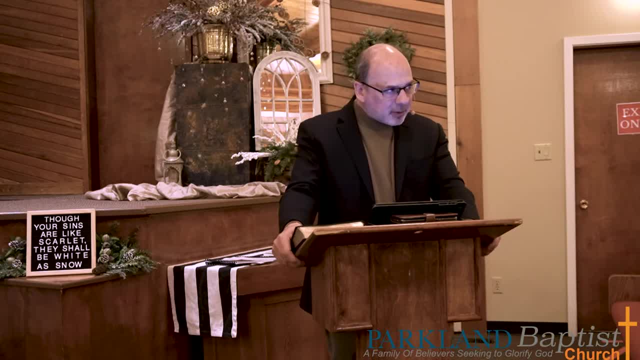 Some forms of theology, such as replacement theology, for example, has to use to some extent a spiritual or a allegorical method of interpretation. They have to. They have to start messing around with some terms in order to justify a system of theology called replacement theology. 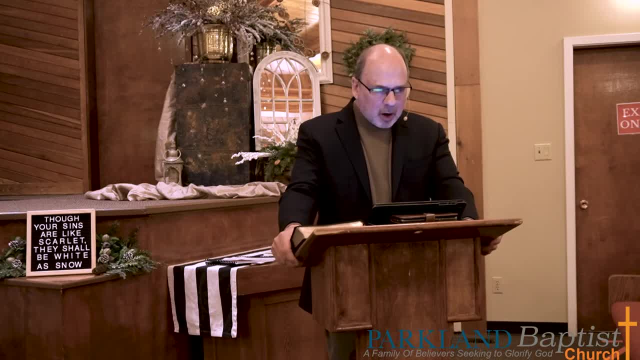 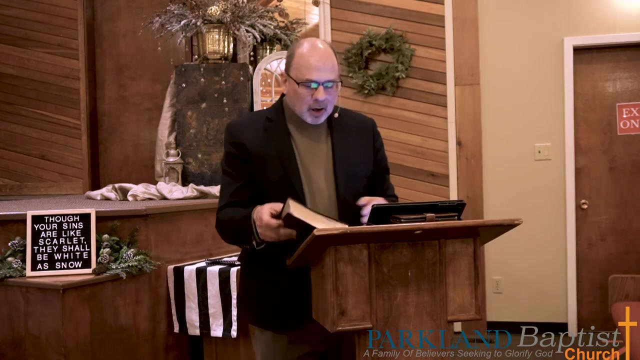 Not all replacement theology. people interpret all of scripture allegorically, but they do interpret some of scripture allegorically, especially the scriptures referring to the end times. So for example, in replacement theology, if one holds to replacement theology, the position of scripture where we are on the prophetic timetable, 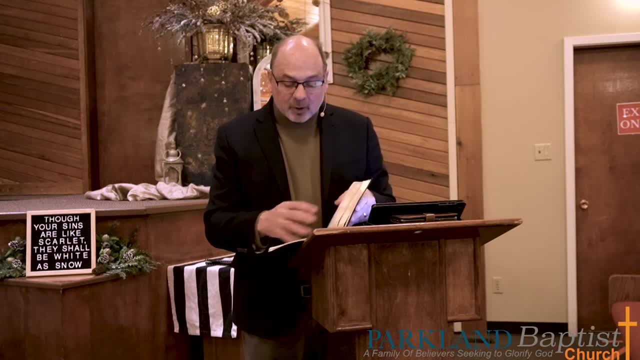 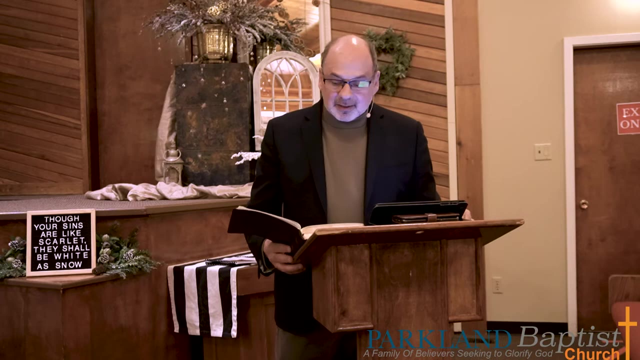 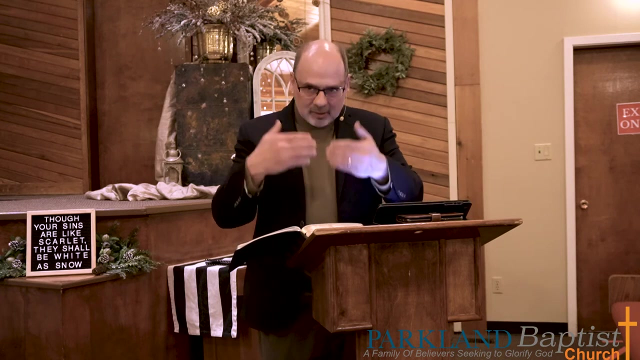 we are now in Revelation, chapter 20.. Okay, that's where we are if we believe in replacement theology. So everything prior to chapter 20 has already happened. It's history, not prophecy. In order to come to that conclusion, you have to start interpreting the text in a non-literal way. 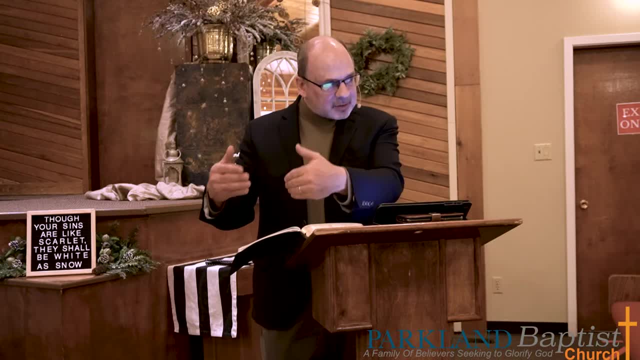 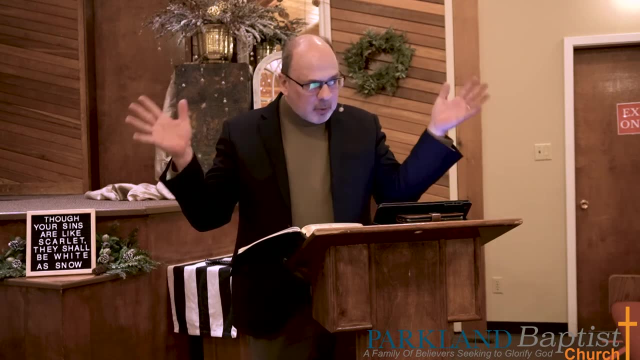 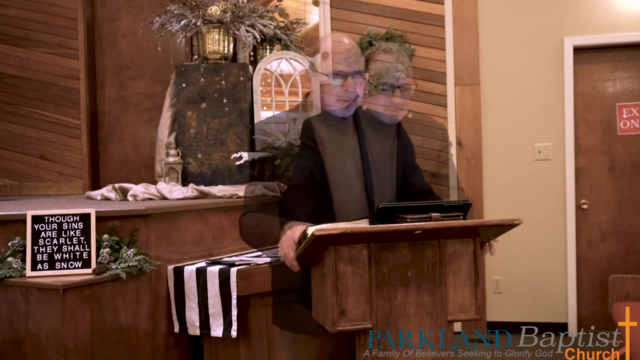 And the way they justify that non-literal interpretation of the text is because the text is so symbolic. Therefore, because the text is so symbolic, we don't know what the literal meaning of it is, so we're going to use an allegorical interpretation to it. 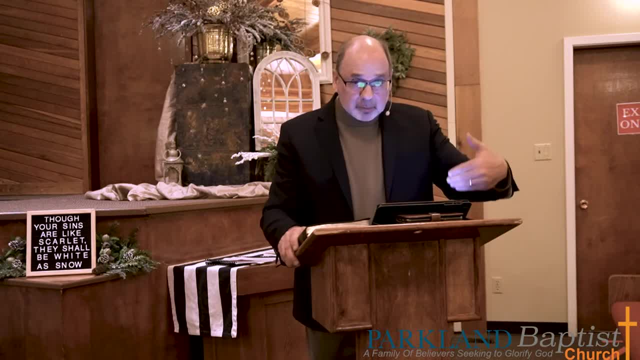 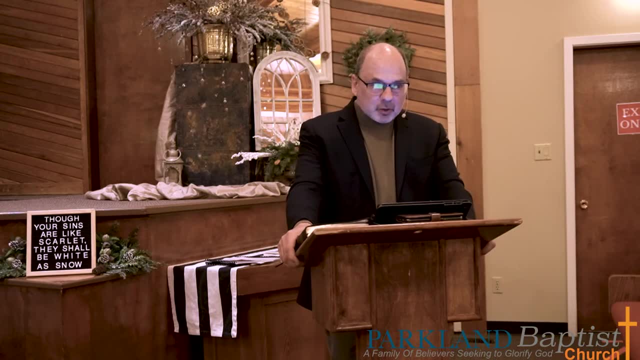 So replacement theology being amillennialism. Amillennialism means It means that we are in the amillennialism, the church age is the amillennial age and therefore Revelation 20 is where we're at. We are living in Revelation 20 according to the amillennialist. 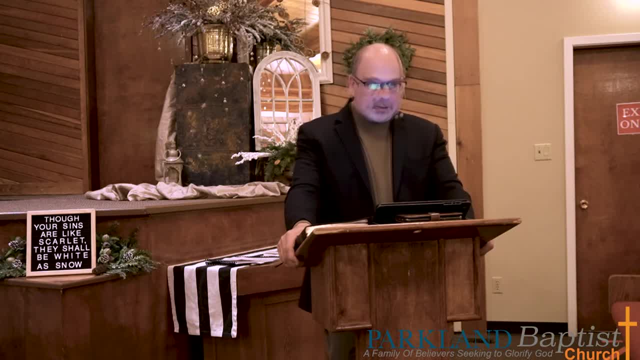 Revelation 4 to 19 is history. Okay, Paul, you had a question, So maybe I'm not quite understanding, but I thought I heard you say spiritual and allegorical. Pretty well, the same thing. The same thing, Yeah. 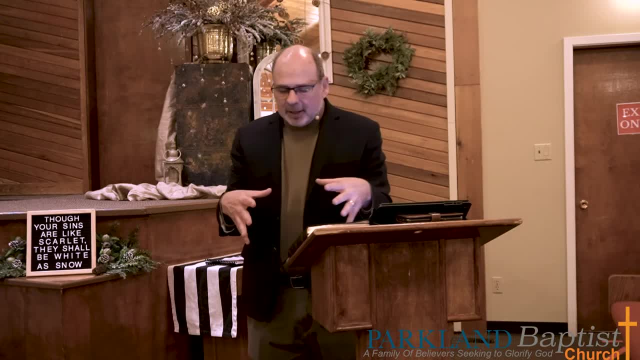 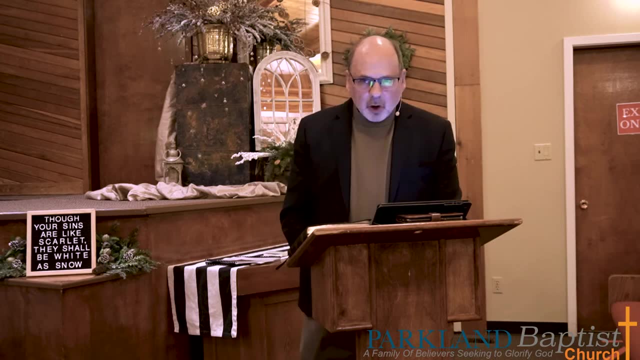 So you're not. you're not limiting your interpretation to the literal meaning of the text, You are spiritualizing it, Spiritualizing the allegorical meaning. So- and you see it mostly happening in prophecy- You'll see this method of interpretation more most frequently in prophetic verses. 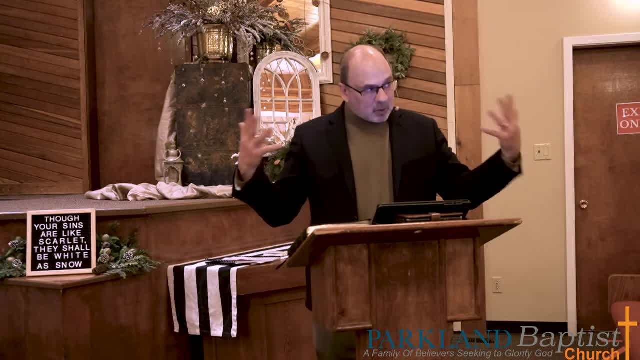 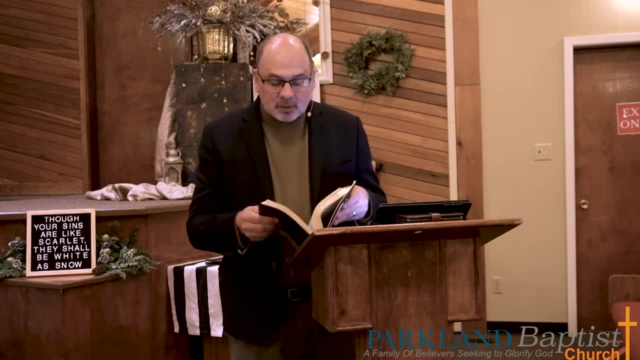 especially prophecy that has not yet been fulfilled, at least according to some. Okay, so another example would be: if you go to Ezekiel, Okay. so another example would be: if you go to Ezekiel, Okay, so another example would be: if you go to Ezekiel, 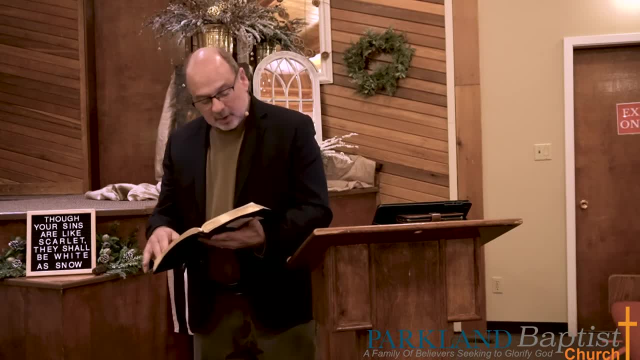 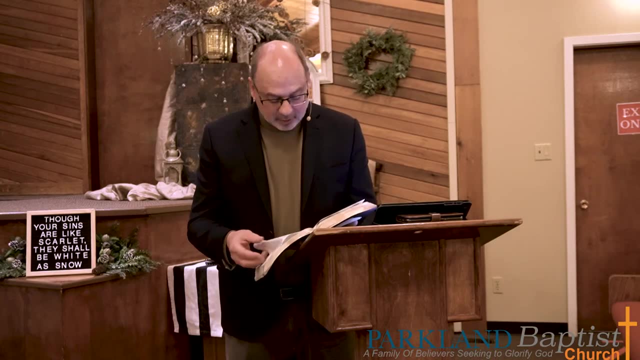 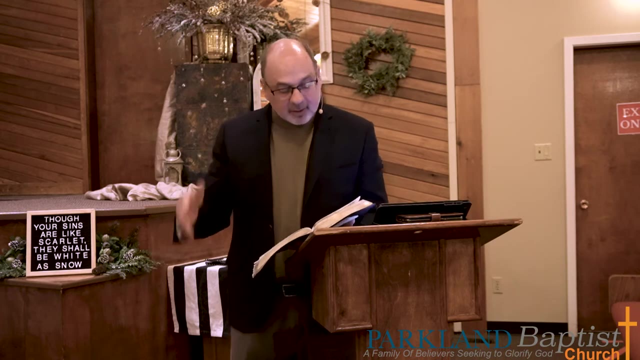 40. Here in Ezekiel, 40 is a prophecy about a temple, from 40 to verses 44, it's the first, or even even more than that, Most of most of chapter, most of the 40s in Ezekiel. 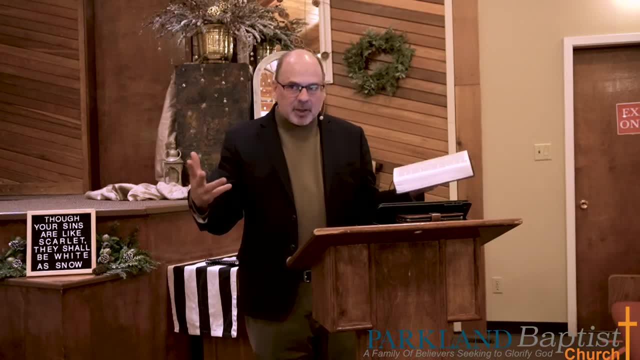 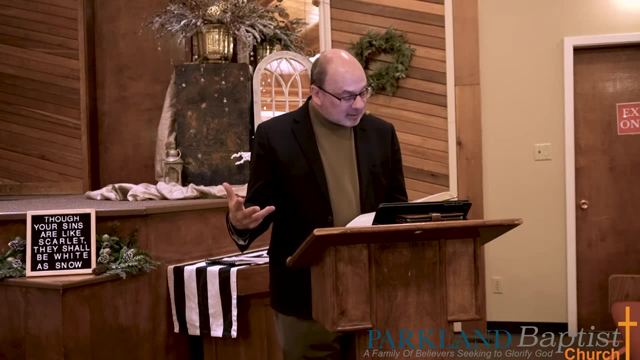 It's about this temple that is being built in Jerusalem. So for amillennialists, they look at this and say, well, there's a temple, There's no temple. Jesus destroyed. you know, the temple was destroyed 70 AD. 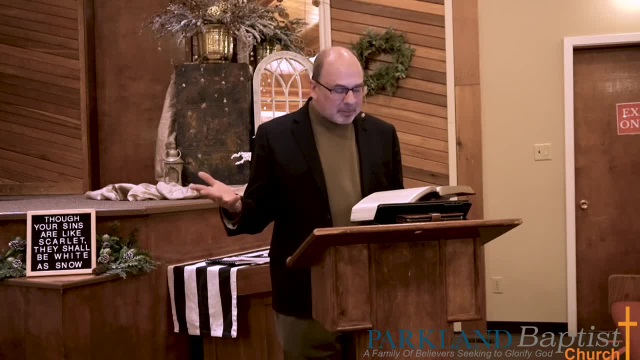 We are the temple of the Living God. there's going to be no future temple. What's this temple about? There is no future temple. There are no future sacrifices. It's over. There's sacrifices in this, So their eschatology forces them to spiritualize these chapters. 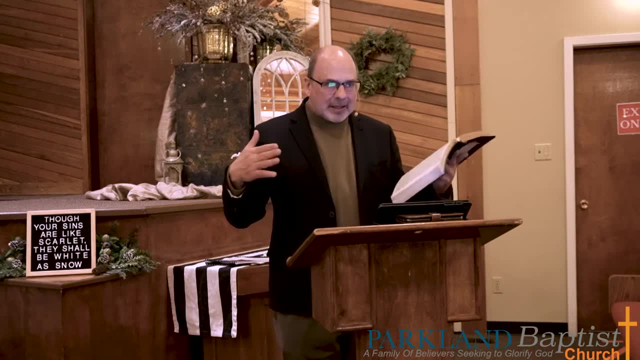 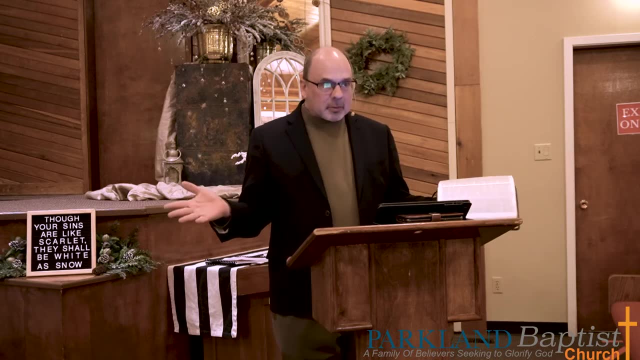 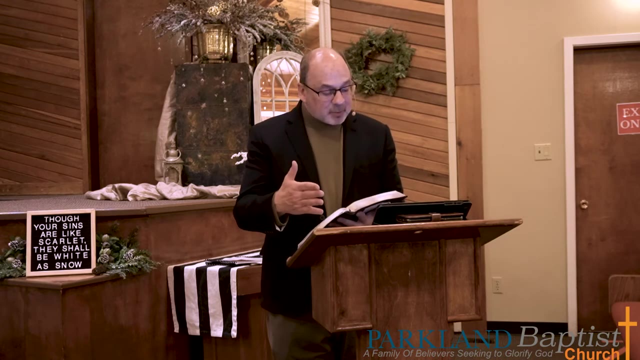 They do not believe that their these chapters are referring to a literal temple that will be built in the Millennial Age. First of all, we're in the millennial age, so that's the one. So all of those chapters, though if you read them they're very specific. 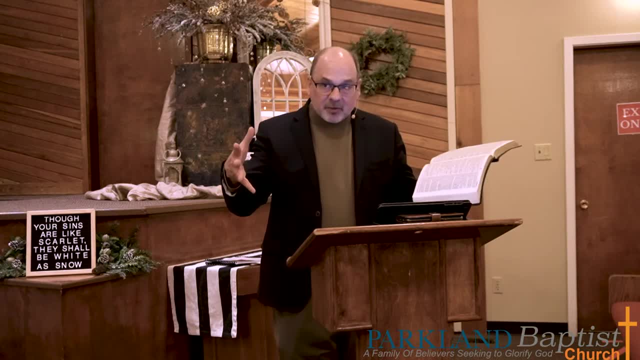 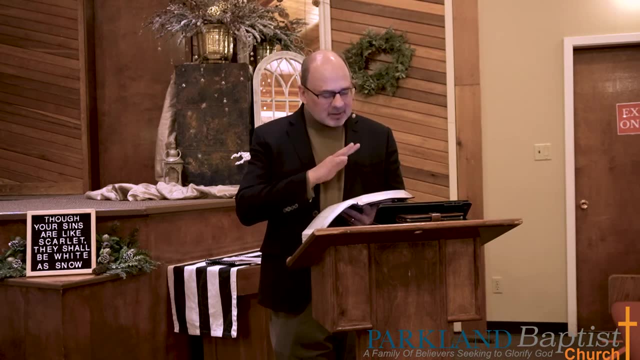 So many cubits this way, so many cubits that way. It's very specific language about the architecture and design of a temple. They don't take it literally Because the literal meaning interferes with their eschatology, And so they go deeper, to a spiritual meaning in violation of what the literal meaning is right. 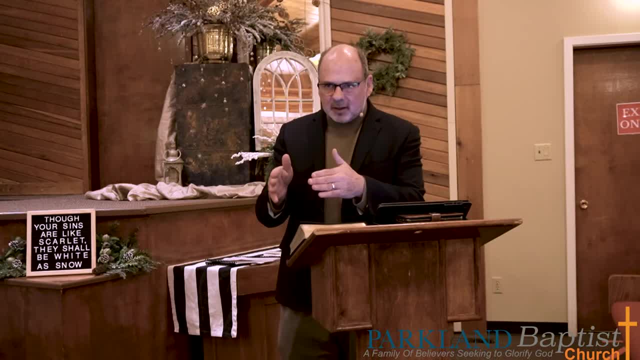 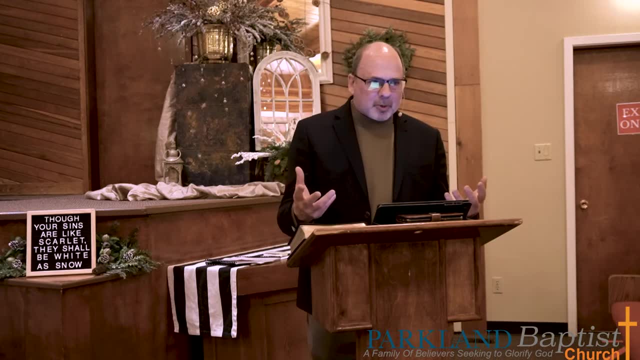 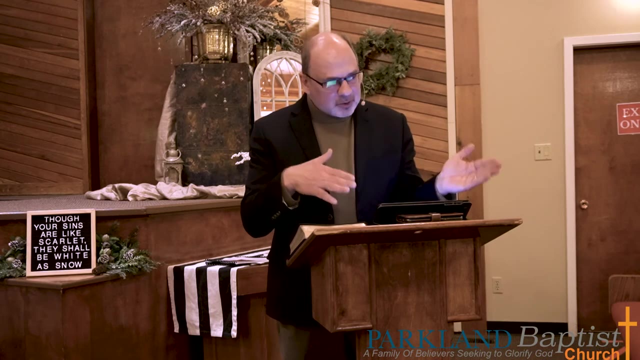 So it's mostly unfulfilled prophecy that falls under the category of allegorical interpretation. They're not going to interpret Isaiah 53 allegorically, because we know how it's fulfilled, But those prophecies that are not yet fulfilled, at least in our mind. 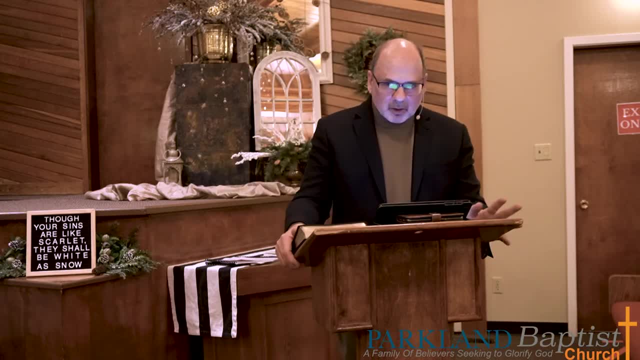 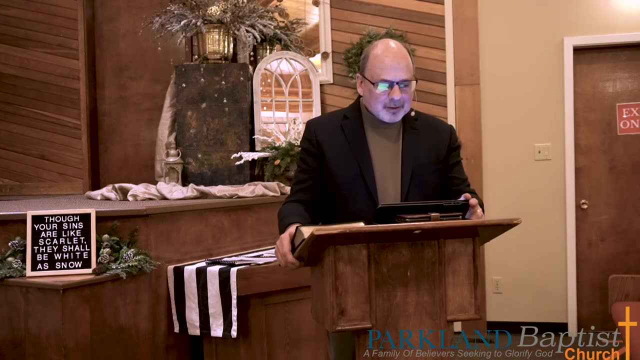 are allegorically or spiritually interpreted. Okay, Is anyone kind of following what I'm getting at here? Just a quick question there: What would you term the temple? I missed that a little bit. Well, Ezekiel 40 to 47,. 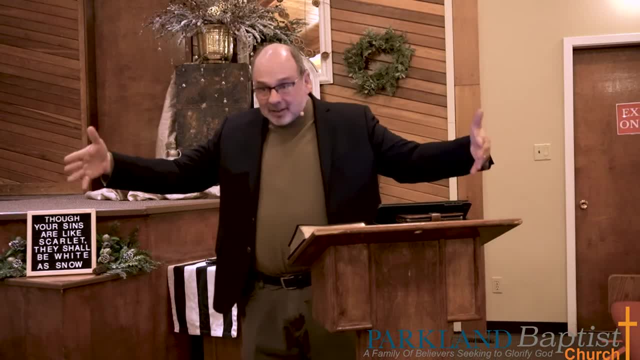 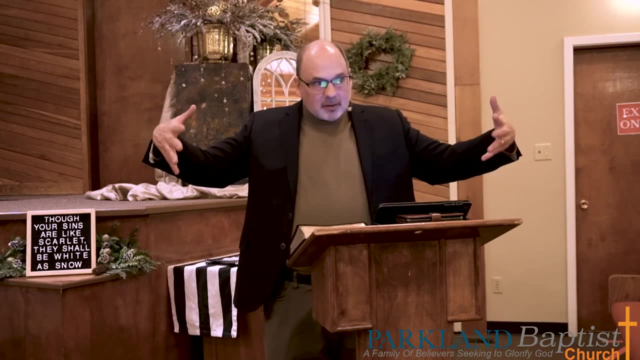 I think that whole those seven chapters are about this temple that's going to be built in Jerusalem, And if you do the, you know, the you know, you say, you study all the architecture of it. that temple has never been built. 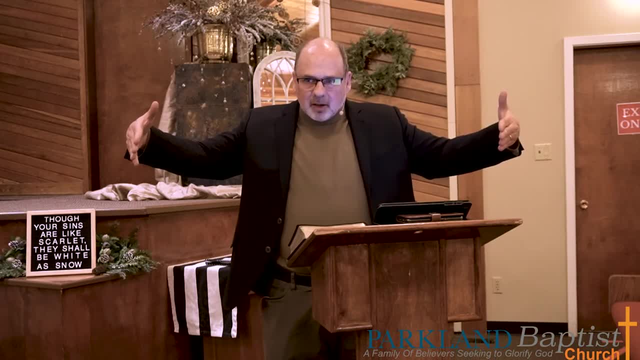 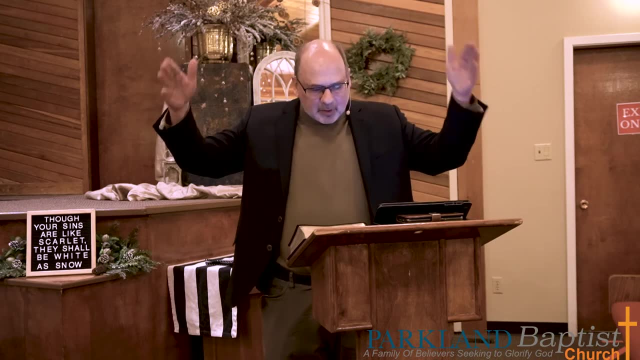 It's a huge temple. It's way bigger than any of the temples that have been built. So most pre-millennial scholars will say that temple is going to exist. during the millennial age, During the thousand year reign of Christ, that temple will be built. 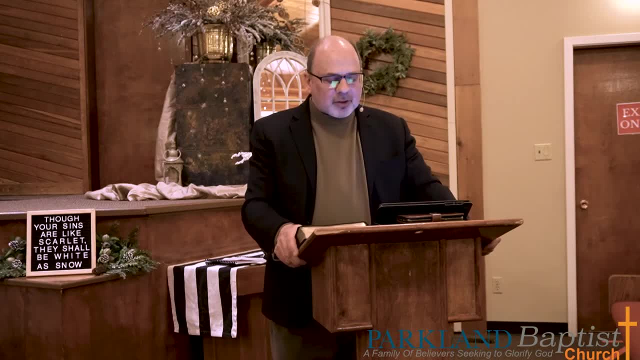 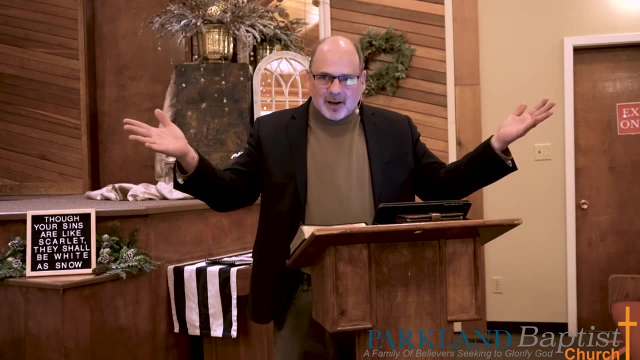 So sacrifices will be done during the millennial age. Okay, So then you see that. So this is the question. So that's a that's an important question. I thought Jesus did away with the sacrifices. Why are we having sacrifices again? 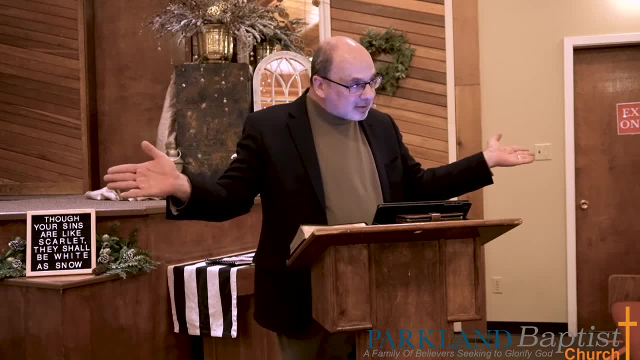 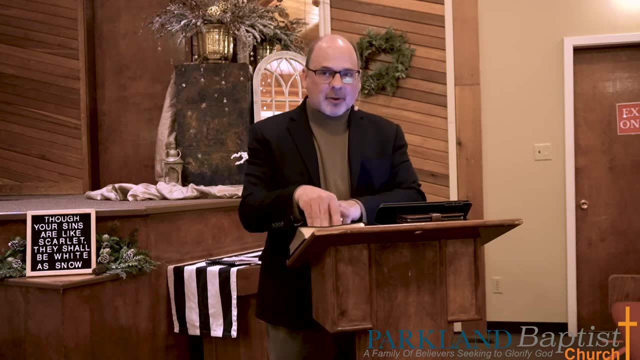 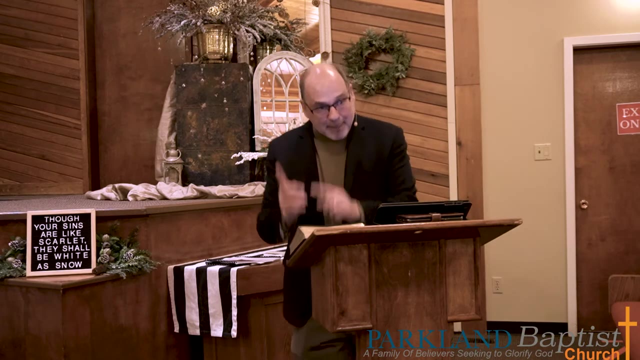 So the way that they would interpret it is because there's no more sacrifices, there's no more temple. This cannot be literal, That has to be spiritual, And so we give a spiritual meaning to it. Well, so the literal meaning is that, just as we celebrate a communion to point back to the death of Jesus, 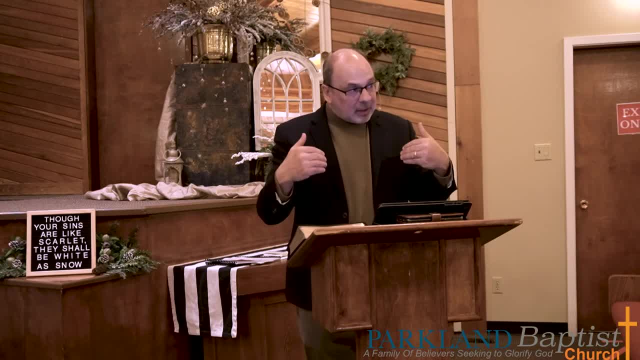 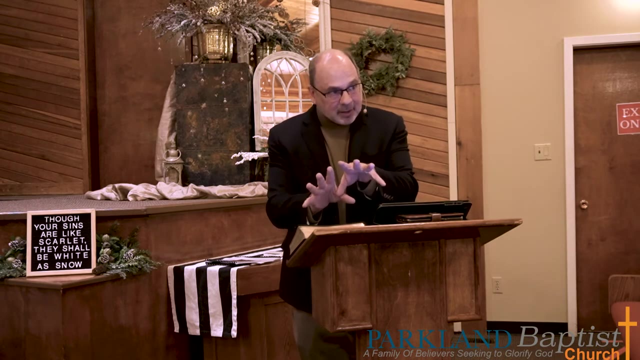 these sacrifices are going to be memorial, not atoning. So there is no atoning sacrifice. If you actually read all the sacrifices, there is no atoning sacrifice. So the thinking is: is that they're going to be memorial? They're going to be pointing to a sacrifice that was made at some point in the past. 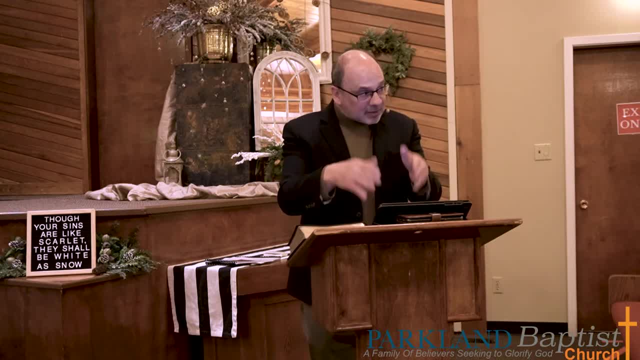 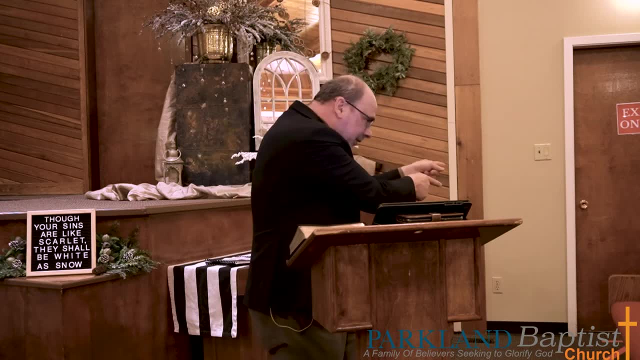 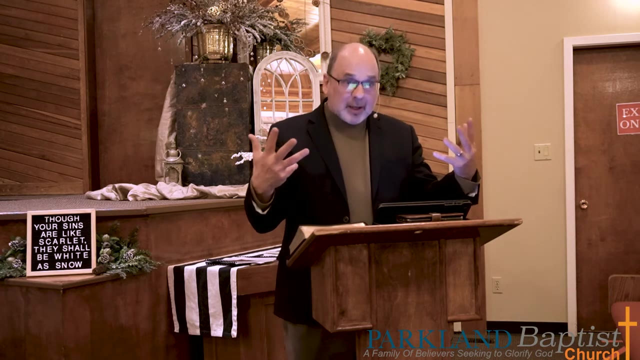 Just like in Solomon's temple, in the tabernacle, the sacrifices were pointing to a future event. These sacrifices will be pointing to a past event, which is- which is the same event- the death of Jesus. Okay, So that's how the premillennial will interpret those passages. 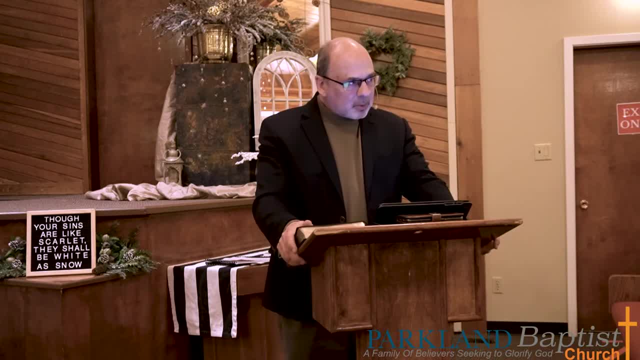 So they honor the literal and they come up with that understanding of it. But if we don't believe in a millennial reign of Jesus, that this isn't church ages, a millennial range, well, you can't literally interpret that anymore. 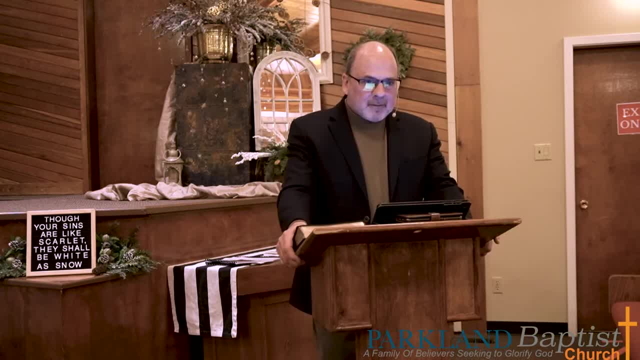 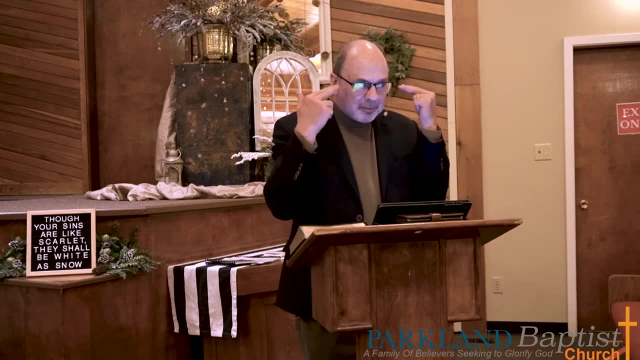 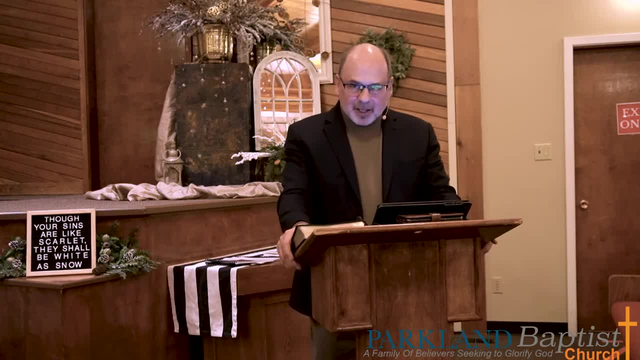 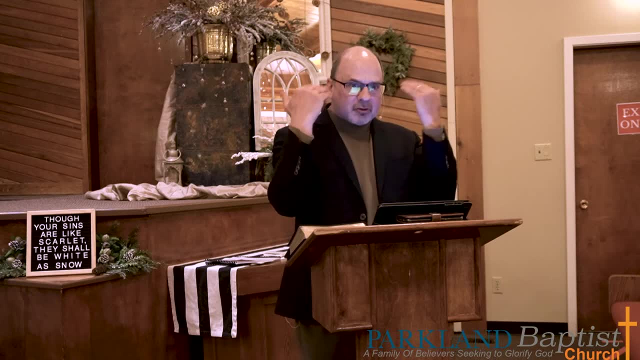 you change the literal meaning to align with my theology. So that's what we mean by I saw Jesus. You're importing into the text of scripture your understanding, rather than allowing the text of scripture to inform my understanding If my understanding is contrary to the literal meaning of scripture. I need to change My understanding, not the literal meaning of the scripture. okay, so what happened? i believe one of the reasons why the church became the new israel is because the early church fathers had a problem with god's enduring plan and purpose with the nation of israel. israel rejected jesus, and jesus and god. 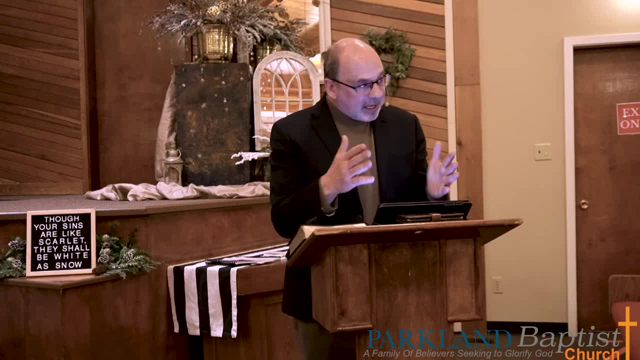 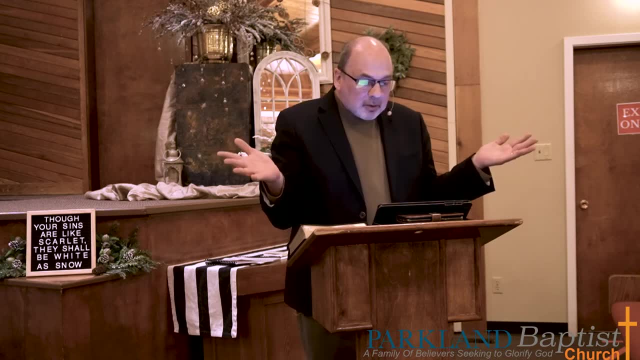 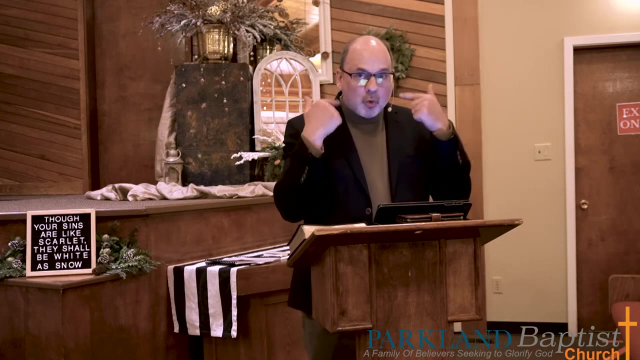 therefore rejected israel, and now the church is the new israel. so they came up with that interpretation because they had a pre-supposition that god was done with israel. so if he's done with israel, then the literal meaning of israel is no longer valid. so they're already. 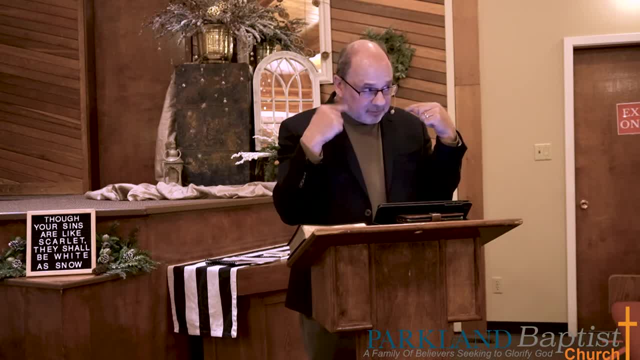 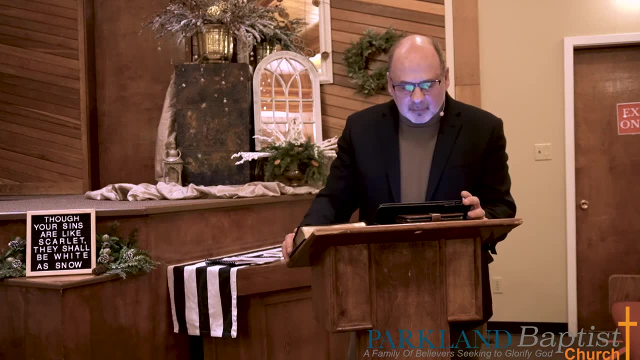 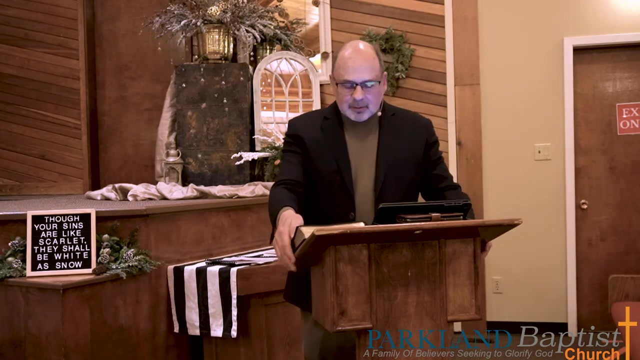 their presupposition forced them to change the literal meaning of the passage. okay, so any other questions? that's pretty important, though, thinking about what you said about, don't let your, your interpretation change the literal meaning of the text. yeah, exactly, we have to let the text change our understanding. that's what it means by being 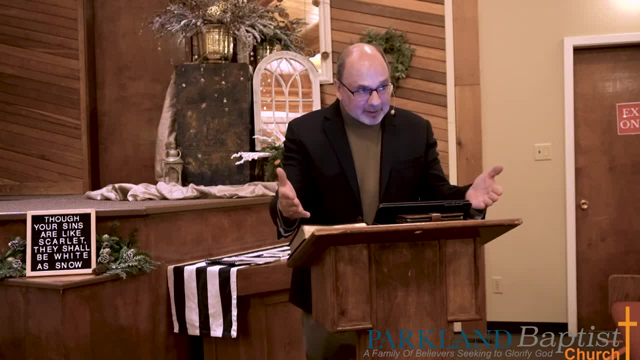 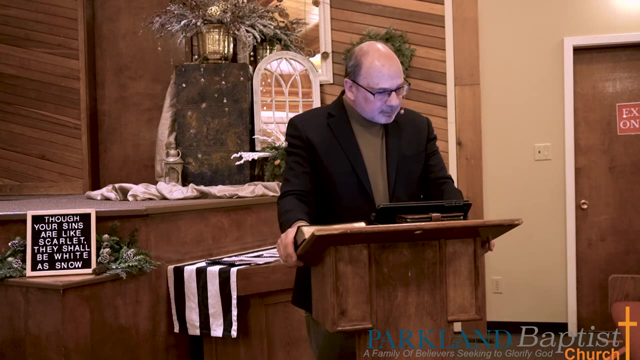 transformed by the renewing of your mind, as you're allowing the text of scripture to correct our thinking. is that why the church has changed so much? um, you know like, uh, through the centuries. you don't like this denomination would be your own denomination, yeah, is that why that has occurred? that i think to a large extent don't agree. 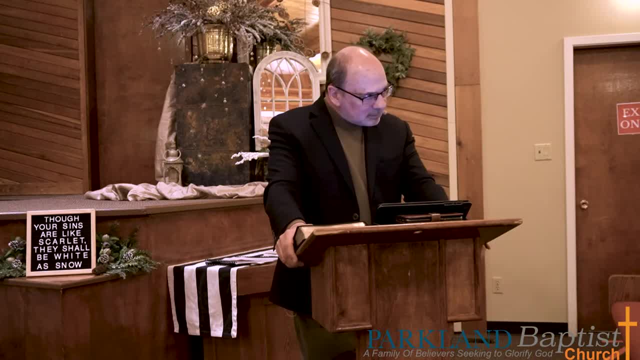 although they're reading the same scripture. yeah, i would think that that's, that's a pretty good assessment. that's why you have like the reformed churches and the lutheran churches and the baptists and this and that because we all come to a different understanding of what the 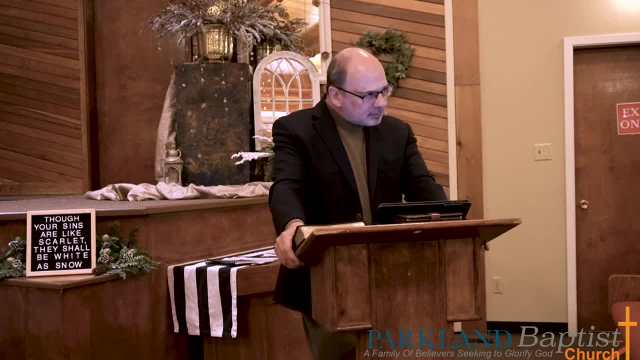 the passoverian church is and the lutheran church is and the orthodox church is and the evangelic church is and the lutheran church is and the lutheran church is and the station is. is what's clicklingamentos actually this give us? is that just most? 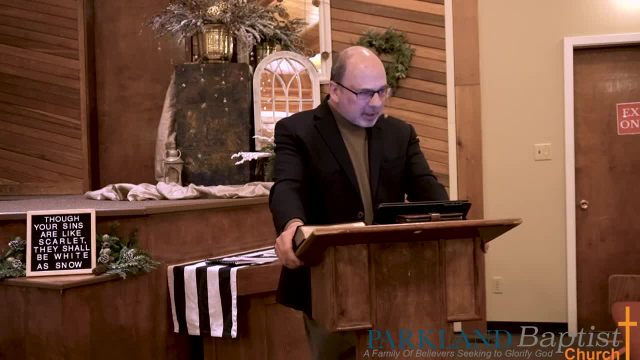 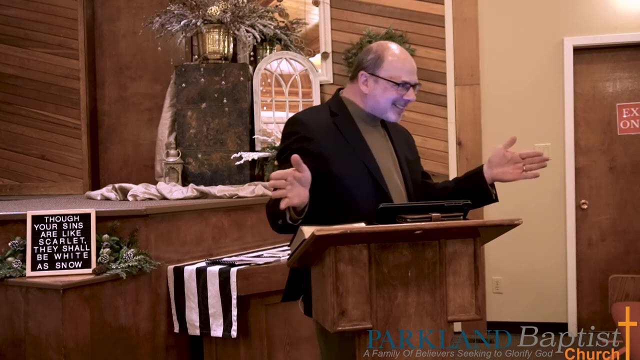 and also well, i would say i would say it. it it's the individual, abruptly nearly gentlemen has brought. it would be sort of a you without disfetish, mostly it more. three to cause: wake up and understand what is this Fundamental King James Baptist people. 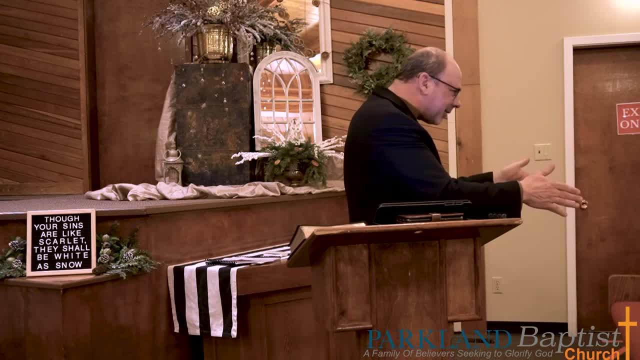 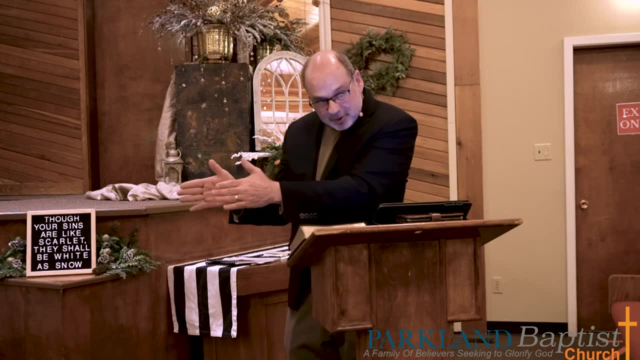 You know we hate gays and we hate everyone and we're going to kill anyone, that's whatever, The real strong, fundamentalist Baptist. Okay, Then you get the other Baptists on the whole other stream, where they're totally liberal, where they're not even believing in Scripture. 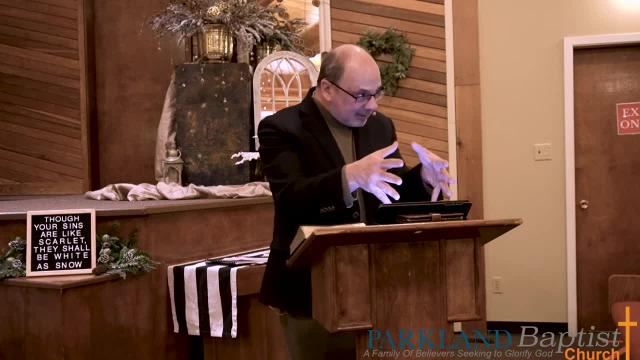 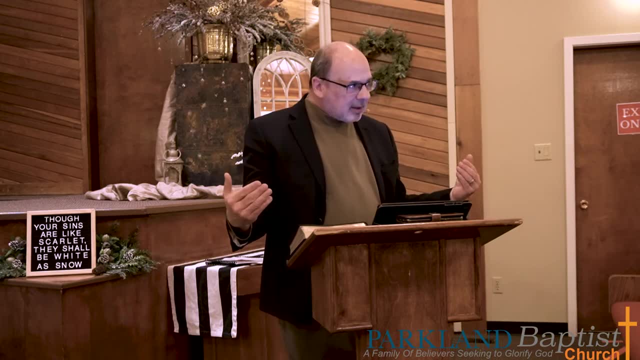 And then you get the middle-of-the-line Baptists, which is probably where we land, where we are event. So even Baptist is a big category, Because all Baptist means really is that a Baptist is one who believes in believers, Submersion. 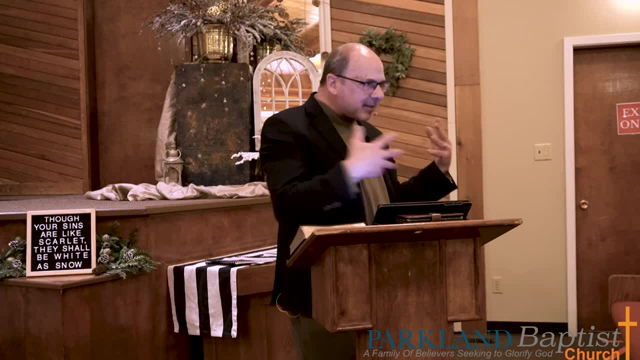 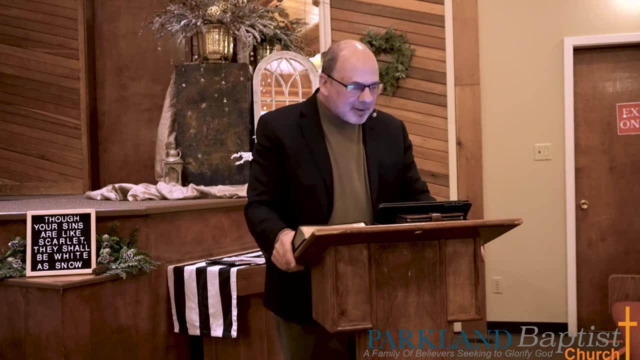 Baptism: Immersion Believers, Baptism- Yeah, That's basically what a Baptist is. Well, that is the truth In terms of baptism. that's the true way. Yeah, On the Baptist. Yeah, Well, yeah. 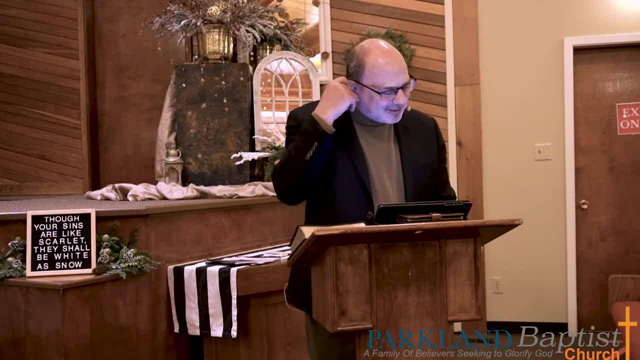 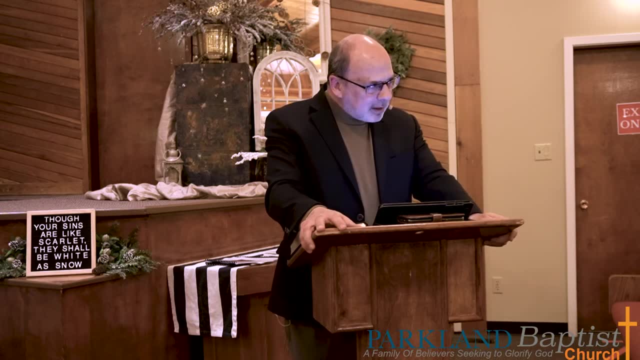 He baptized with water, but Jesus baptized with the Holy Spirit, Right? But the statement of Chicago- do we believe this here in this church? Yeah, That's what it says. Yeah, Mostly or mostly. Well, the leadership does Okay good. 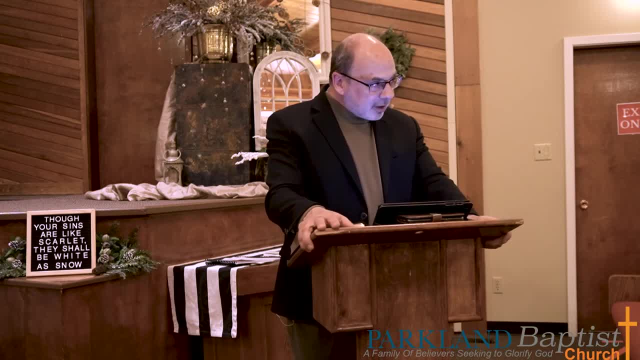 I mean, we have no control over you know people's individual theologies, but the leadership believes in those statements, Absolutely Okay. Yeah, That's where this church would stand with respect to the Scriptures. I might be here for a while. 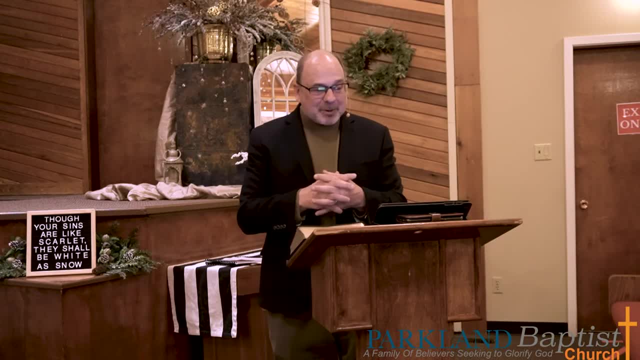 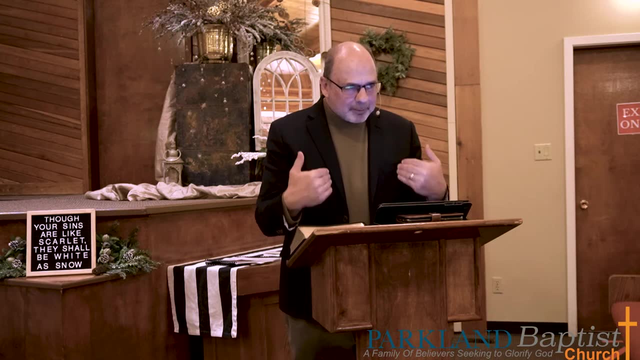 Okay, so here we are, The literal method. The first thing is understand what it meant before we ask how it applies. Okay, This is what we call the exegetical statement. We have to. We have to understand what it meant to the original authors. 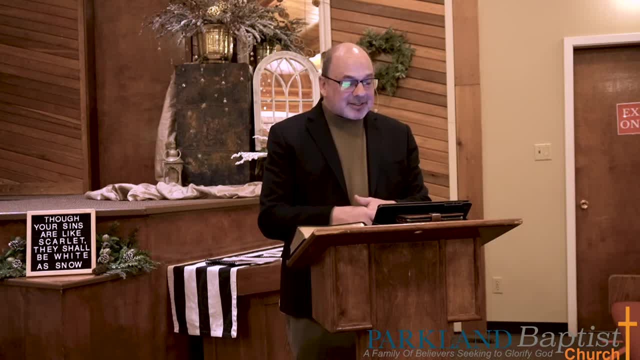 You know I've been to many, many Bible studies, I've led Bible studies, I've been in Bible studies And this is sometimes how it works. People you know read a passage of Scripture. Let's say: we're studying, you know Romans, whatever. 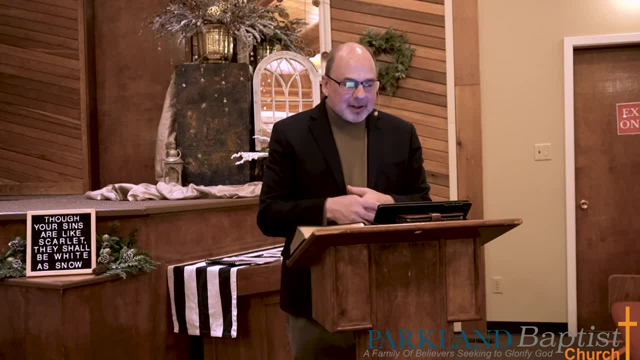 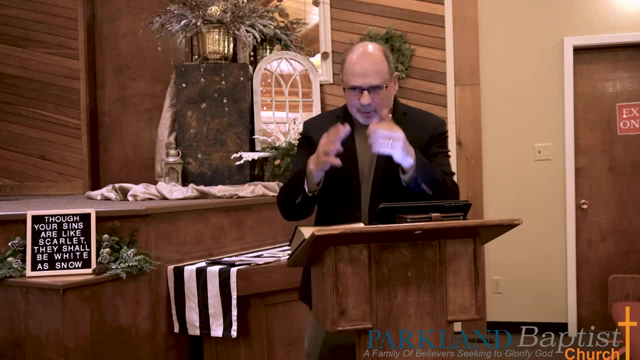 Okay, So we read Romans, 3, chapter, verses 1 to 10.. So we read the passage and then the leader goes around. Oh, John, what does that mean to you? John gives you his interpretation. Sally, what does it mean to you? 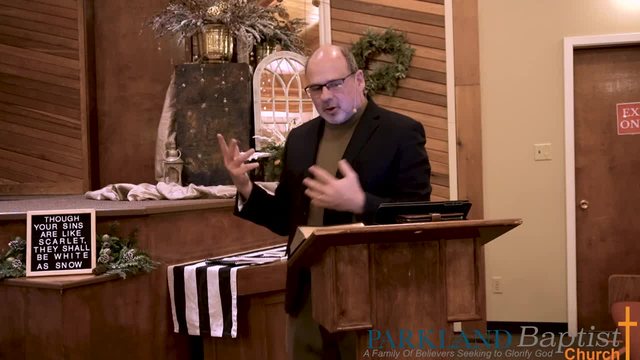 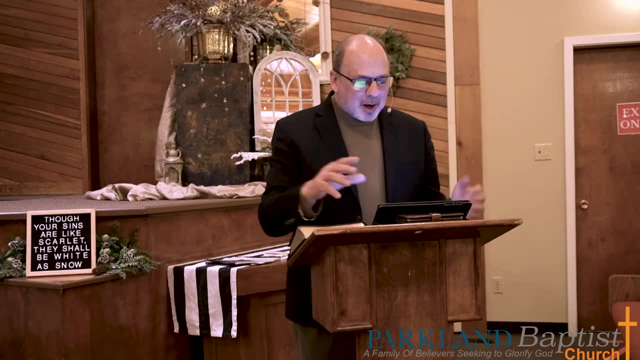 Sally gives her interpretation. And then, George, what does it mean to you? You go around And you have 10 different people giving 10 different meanings. So this is not a proper method. It's not. what does the passage mean to you? 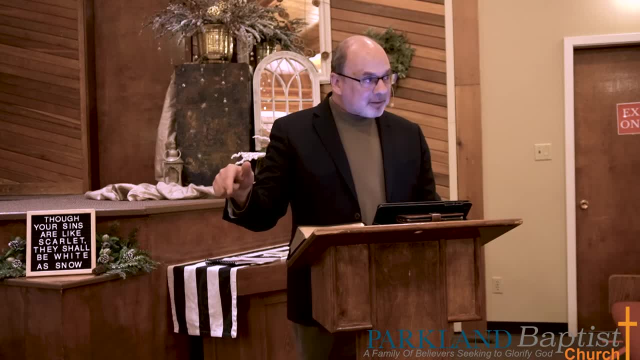 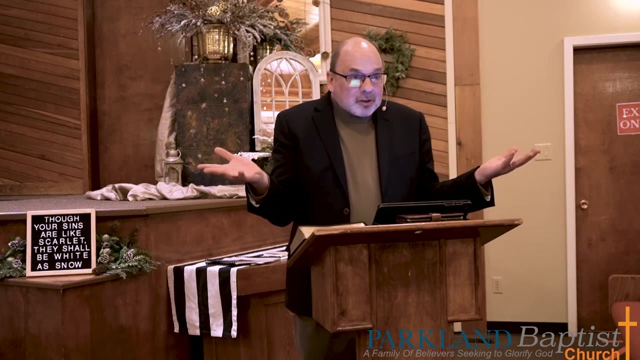 It's. what did the passage mean to the original readers? What did it mean to the original audience? That's how we have to do this, Because we can make it mean whatever we want. For example, what does marriage mean today? What does even biological gender mean? 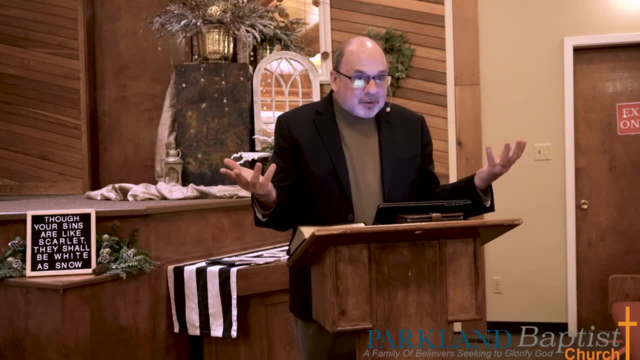 I mean, you look at it, you have how many pronouns. 50 different pronouns for our biological orientation or our sexual orientation. You have 50 pronouns now. 20 years ago I only knew two right, So notice how the meaning changes. 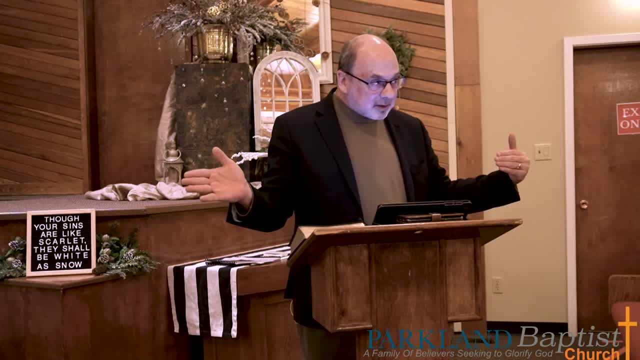 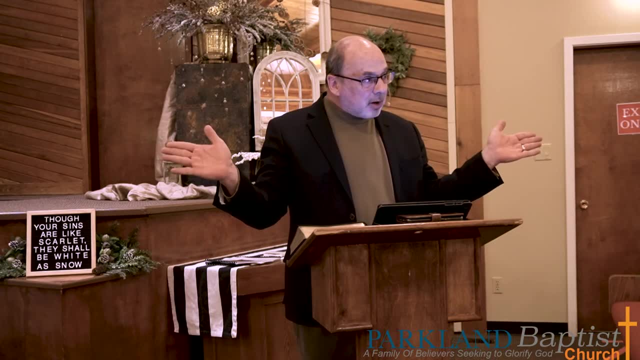 Well, the meaning of marriage is different now. Marriage doesn't mean just necessarily the exclusive relationship between a man and a woman for life. I mean, now the definition is far off, It's far broader. So you see, it doesn't matter what it means to me now. 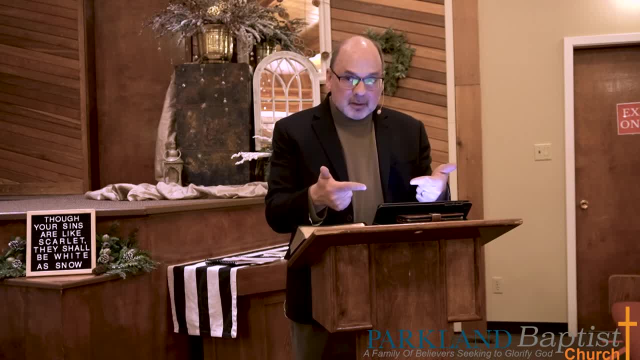 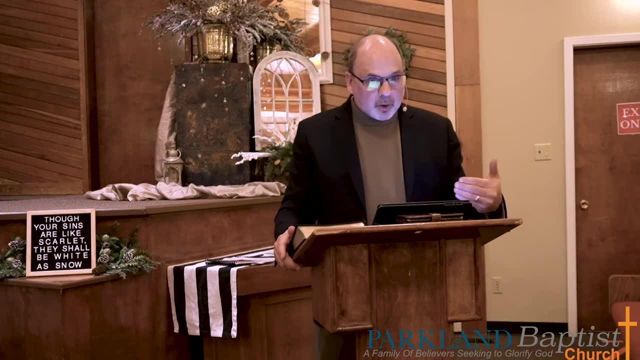 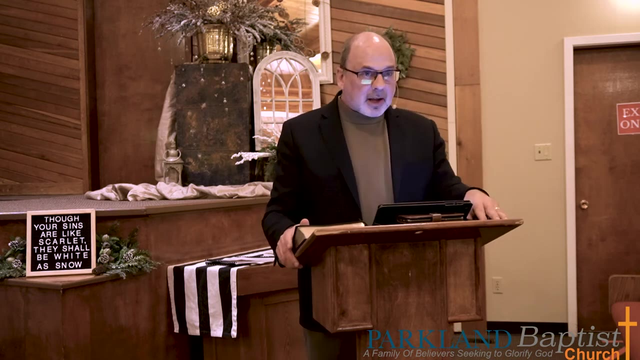 It matters what it meant when it was written, Because the meanings can change over time. Okay, so that's how this works. when we do a literal interpretation of scripture, We have to get at the original meaning of the text, And you can get that using Bible tools and stuff like that. 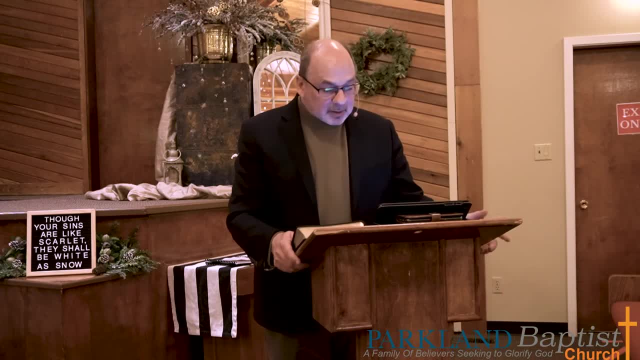 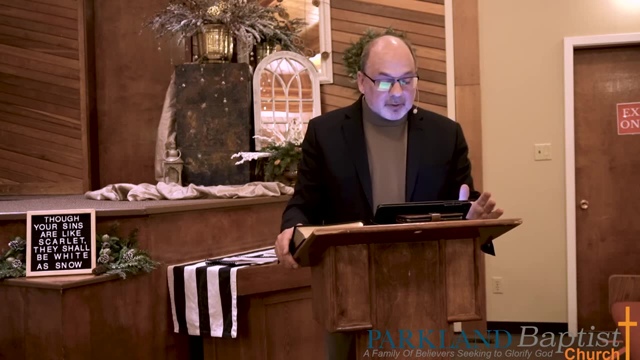 So when we approach scripture, we should not even begin to ask: what does it mean to you? What we have to always ask is: what did it mean to the original audience? The reason we have to do this is because the Bible was not originally written to us. 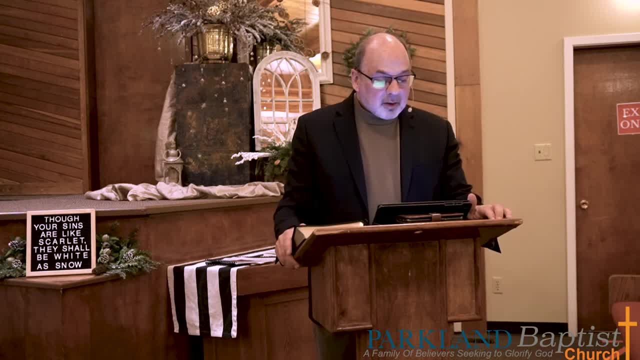 but it was written for us. Okay, The Bible was written to an original audience, to the Church of Philippi. It was written to the Philippian saints. It was written to the saints of Corinth. It was written to a particular audience. 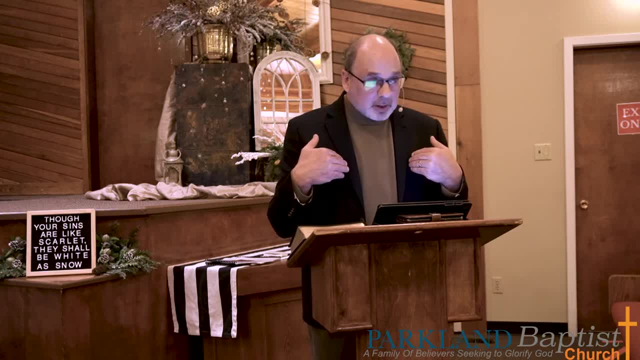 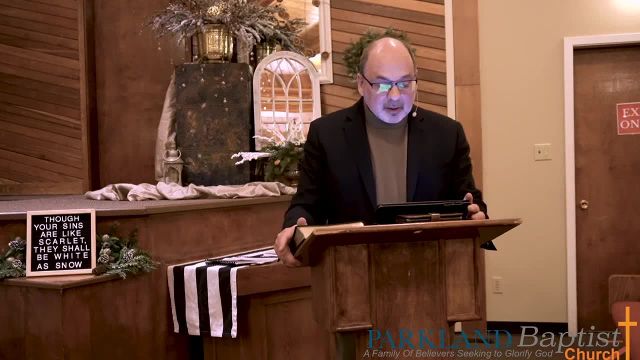 So it wasn't written to us, but it was written for us. We derive benefit from it, But only in so far as we understand what it meant when it was written at the original time. So what our job to do and what our job is as interpreters of scripture. 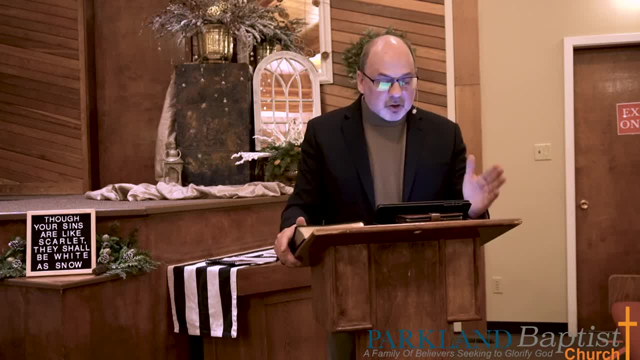 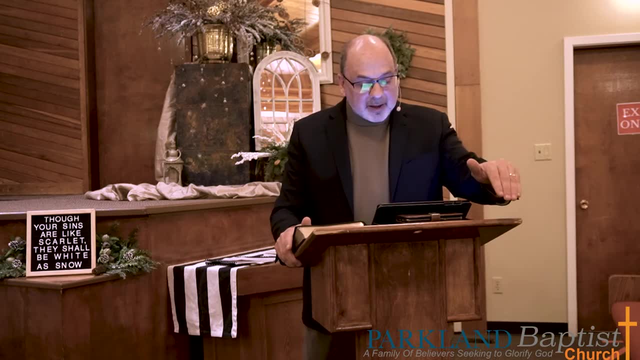 and we can all do this because, like I said, there's tons of tools around to do this. Our job is to overcome the hurdles of time and faithfully understand what the passage meant to the original audience. Okay, And then, once we understand that, we come up with it. 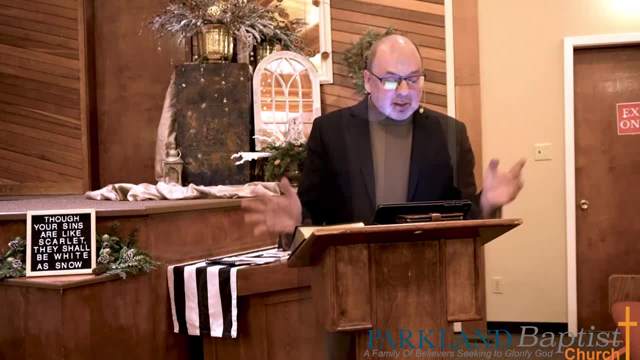 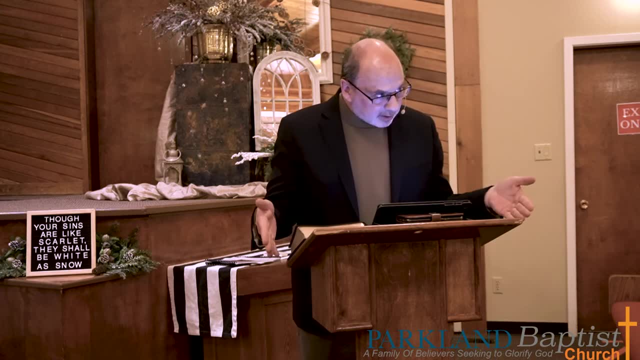 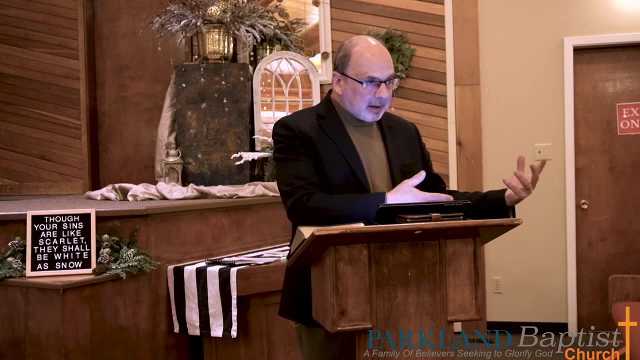 And then, once we understand that, we come up with an application for today. Okay, Generally- and I'm saying generally- a given passage of scripture has one meaning, And that is the literal meaning, But it will have many applications. In other words, there's various ways we can apply that particular meaning of scripture. 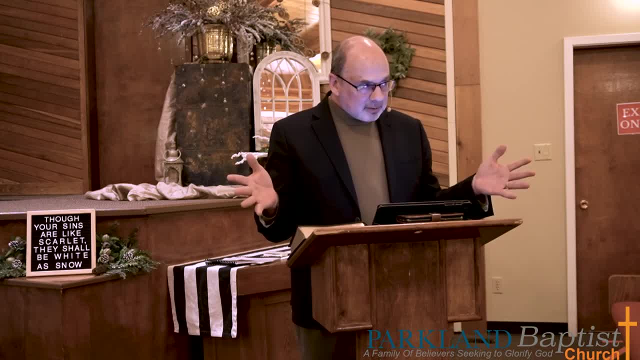 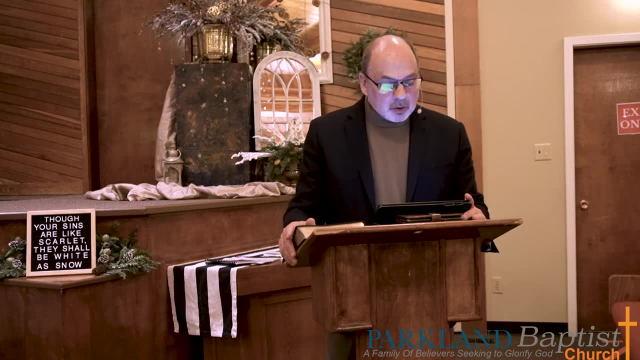 There's many, many ways to love your neighbor. That's the application. I gave an example there, but we're running out of time So you can read through that example. So step one, then, is to understand what it meant then. 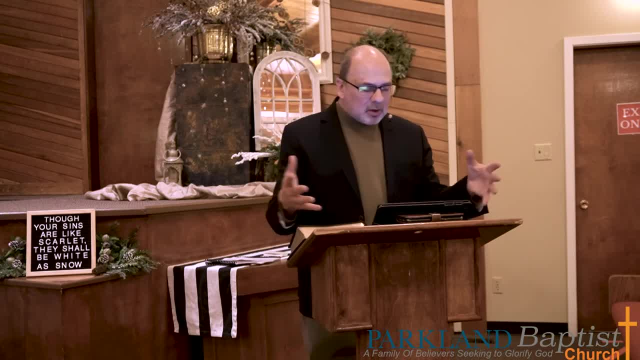 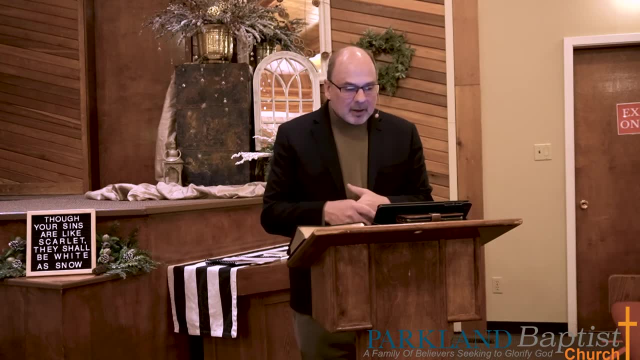 The next step is: what is the timeless truth? So once you get at the original meaning, you want to pull out like the timeless truth, the truth that applies for all time. Okay, And the way you do this is to compare scripture with scripture. 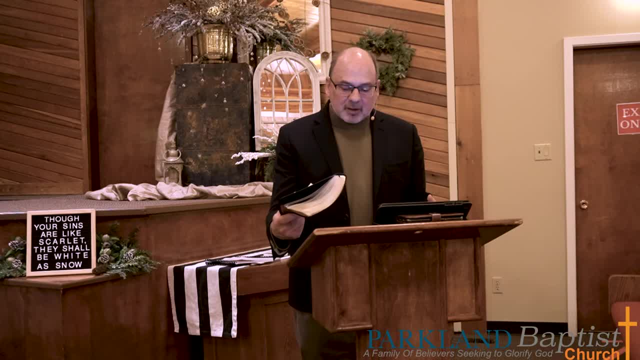 That's a wonderful way, Like I love this Bible here, this New American Standard, because it's got references in there. So basically, When you read a passage, there'll be like an A on there and the A will take it to the margin. 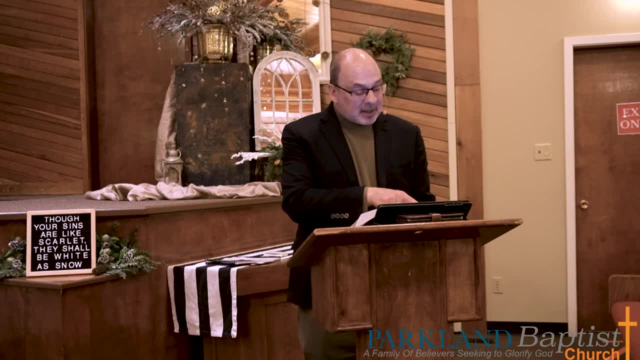 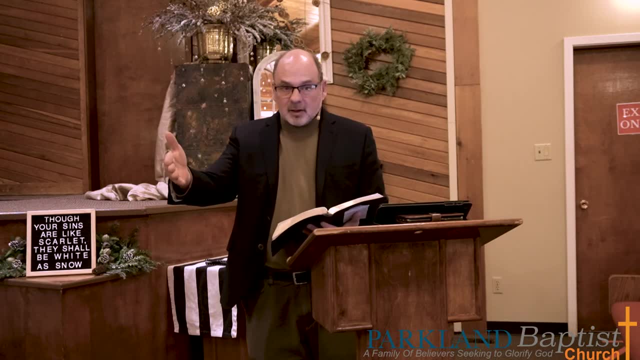 and it'll say: well, these other verses in the Bible have the same meaning or not. the same meaning, the same words? Oh well, that's great. Well, let's see what Isaiah has to say about this. And what does Paul have to say? 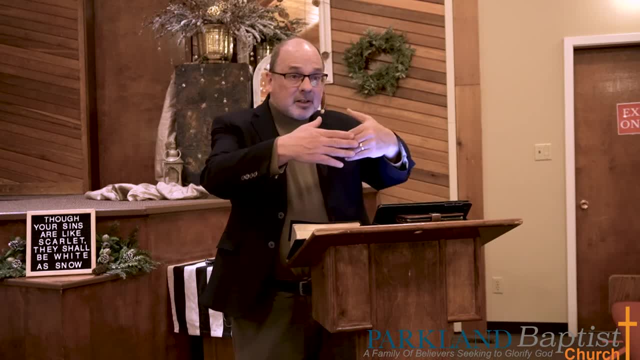 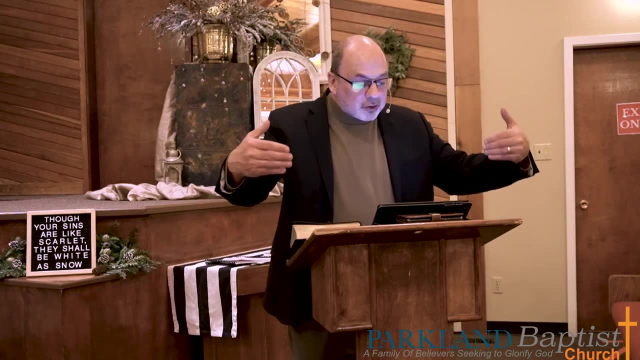 So you compare scripture with scripture, and then you start to get the bigger picture of what the meaning of the text is. So that's the second step. That's where you start to develop a timeless truth, A principle, A principle that transcends time and place. 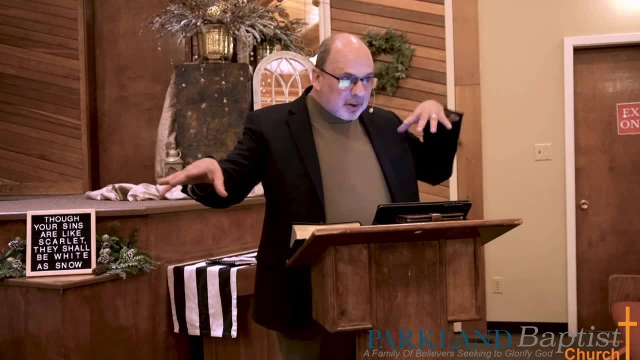 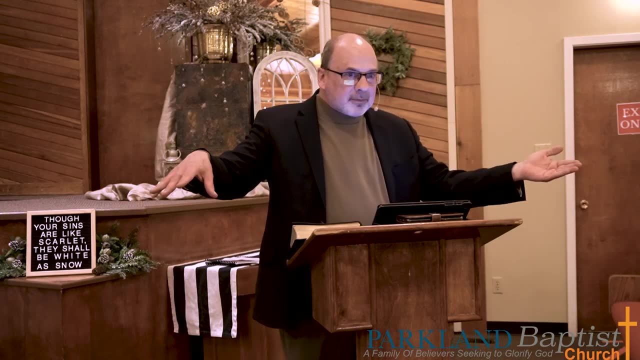 It applies in China as much as it applies in Mexico, as much as it applies in Canada, as much as it applies in Cuba, And it applies in the 21st century as much as it applies in the 10th century. Okay, 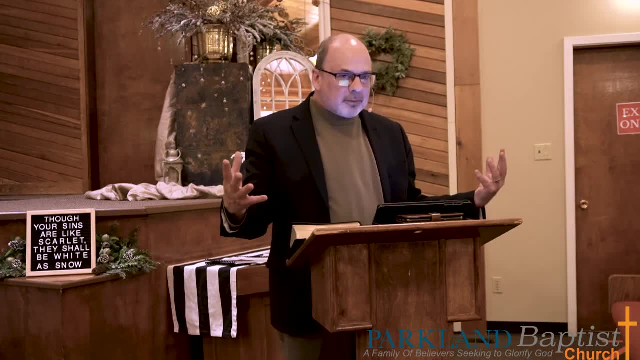 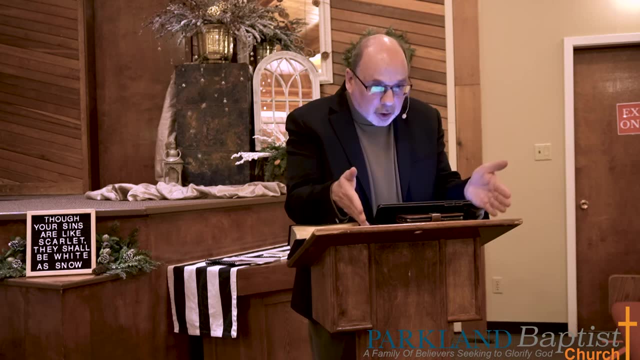 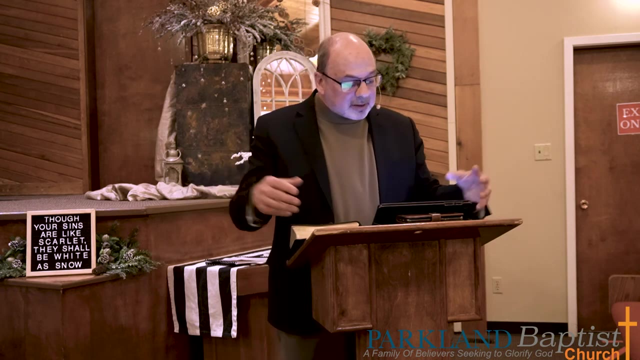 So that's what we mean by the timeless truth. It's universal, A universal truth. The first thing is to understand the original meaning of the passage or of the words. Second, you compare the scriptures with the scriptures To get at the bigger picture, the timeless truths of it. 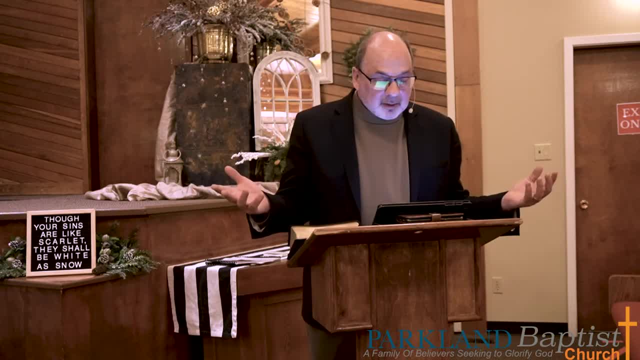 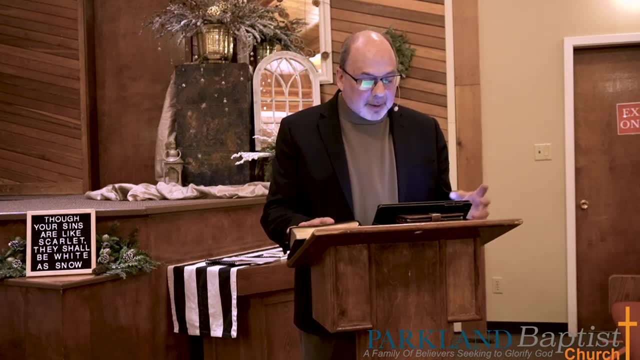 And the third thing is: the third step is then: how do we apply this? How do I apply this in my life? Okay, And that's the application. That's a lot of what the preacher does, right? They extract the exegesis, try to draw out the meaning of the text, find the timeless principles and give an application. 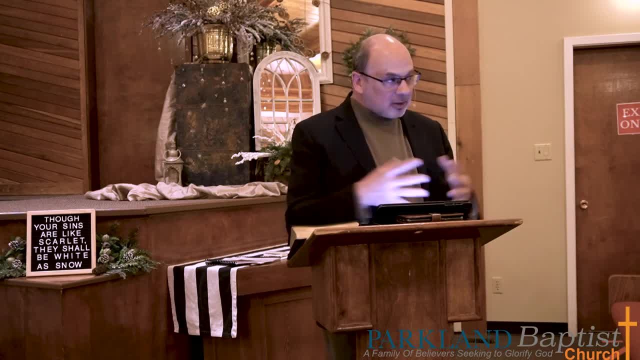 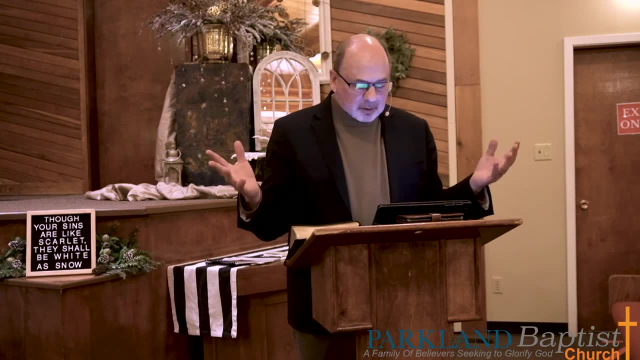 Okay, So we can all do this. You don't need a PhD to do this. Okay, All you need is some good Bible study tools to get at the meaning of the text. The internet's a good place, But watch out where you go for your internet. 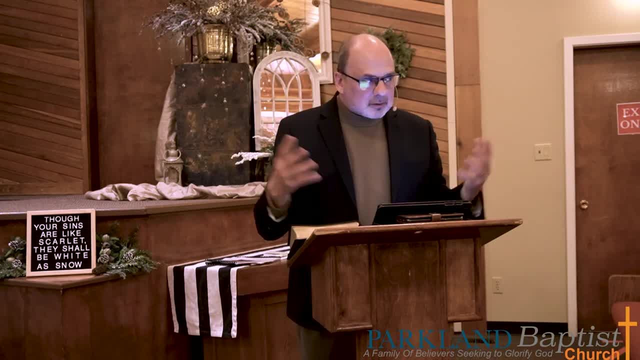 You don't want to go to some wacko conspiracist guy who's you know, always on a conspiracy thing. You want to go to some sound places. Bibleorg is a good place. Precept Austin, I think it's called, or Austin Precept. 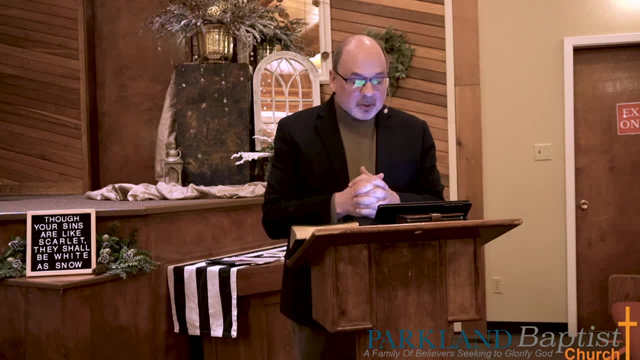 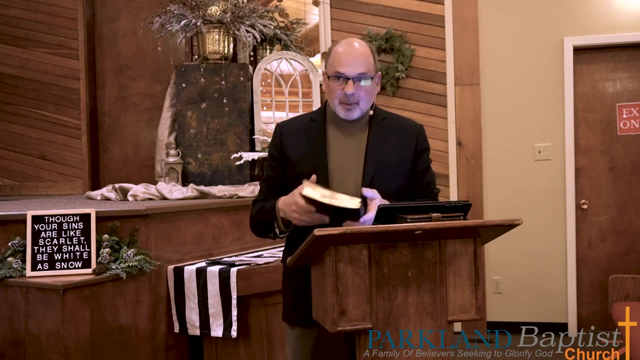 Very good place eSword- if you have eSword You know those are some good basic tools. And then get a Bible that has references on it, a reference Bible where it shows other verses, parallel verses with the same meanings. 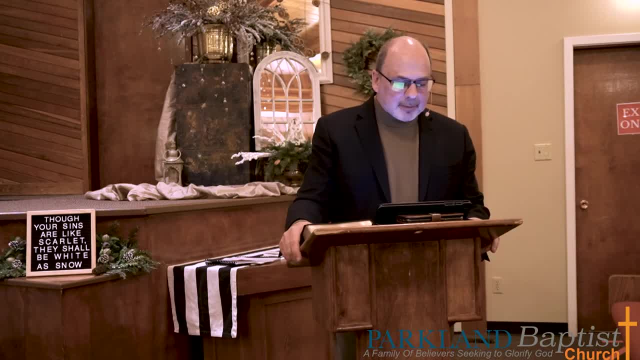 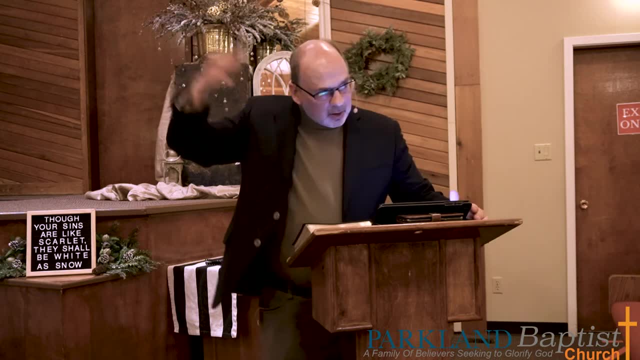 Or Strong's Concordance will do. that's the same thing. you can use that, And then you just search out the different scriptures. This is why when I preach, you know you notice I'll take you to. well, here's the passage in 1 Corinthians, chapter 10,, for example: 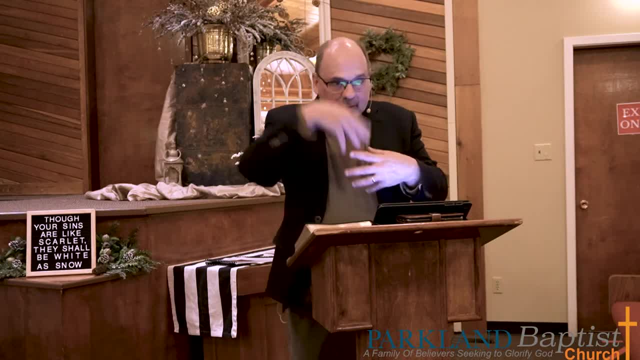 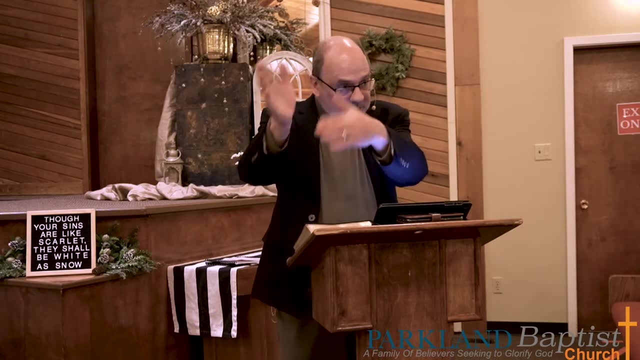 Or here's, you know. so I'll take you to other scriptures, and that's what I'm doing Is comparing scripture with scripture so that we get a bigger picture of what this means. It's not just in Isaiah, it's also in Romans or in Genesis or whatever. okay, 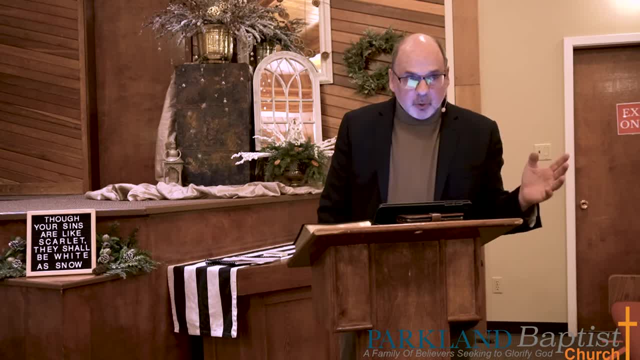 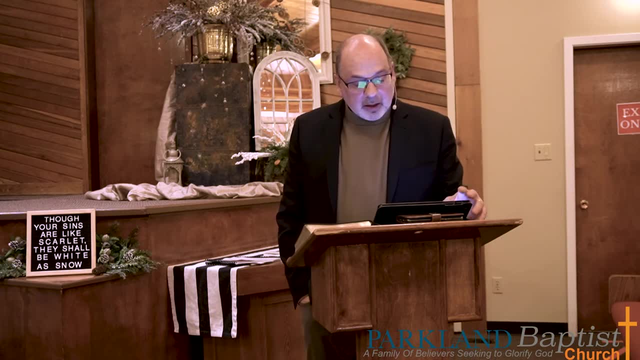 Okay. so once you've done that, then you come up with an application. So a few words before we end here. I mentioned two words already- exegesis and eisegesis- And again I want to just go over what these mean. 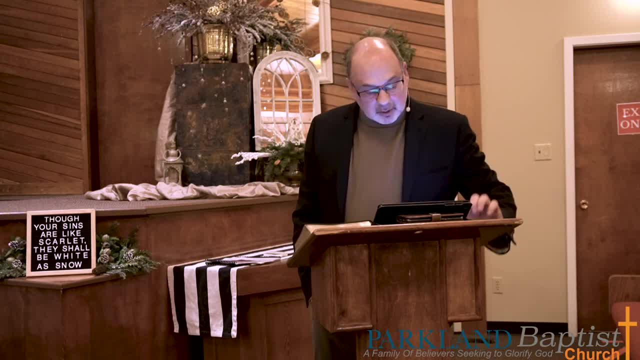 Iso is a Greek meaning into And then exo is a Greek meaning out of. So iso refers to a subjective method of doing theology. Another term we can use is called a reader response. You know, there is a movement that says- and I think I shared this already before: 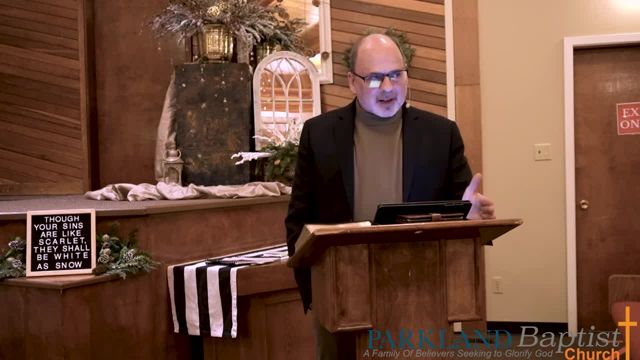 that the reader has the final authority on what the text means. So a eisegesis would be a reader-centered hermeneutic. I determine what the meaning is. The reader has the final authority, not the author. okay, So a reader response has absolutely no concern with the original intent of the author. 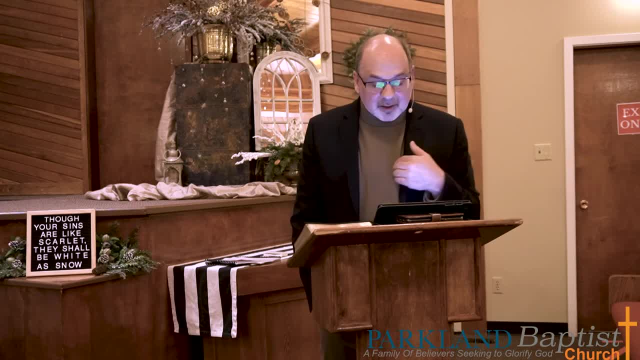 No concern with what the original meaning is. The only concern is what it means to me. That's a reader response And some paraphrases do that. A paraphrase of a Bible like the message. I mean, I understand why people like to read the message. 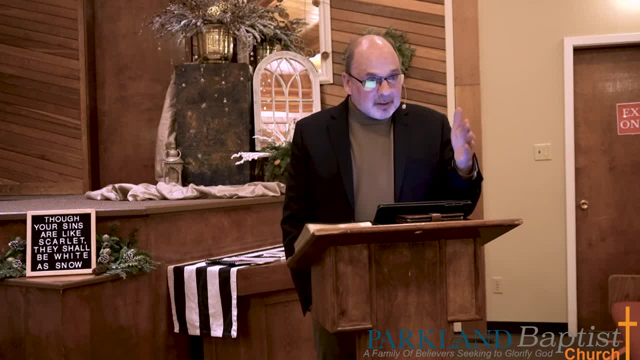 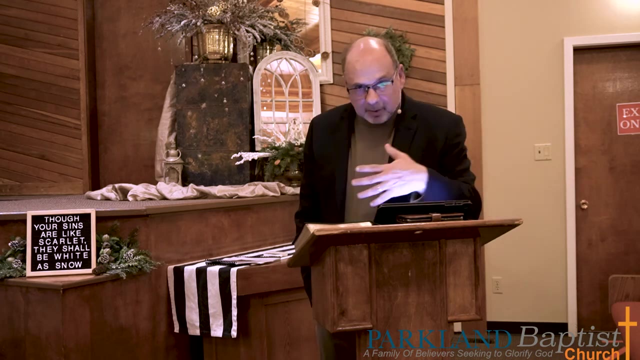 Because it's understandable language, But at The expense of the sometimes the literal meaning of the text. It's a reader-centered paraphrase. It's all about making it readable, Not to say that all of them that paraphrase is wrong. 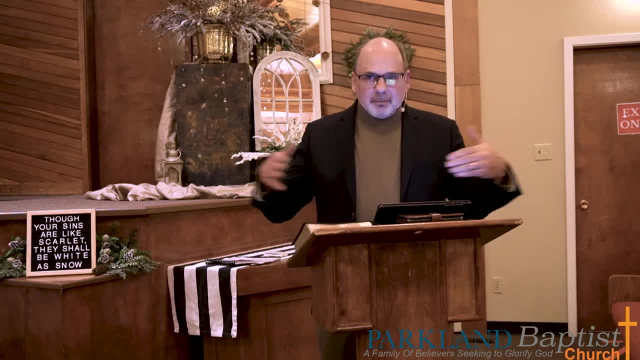 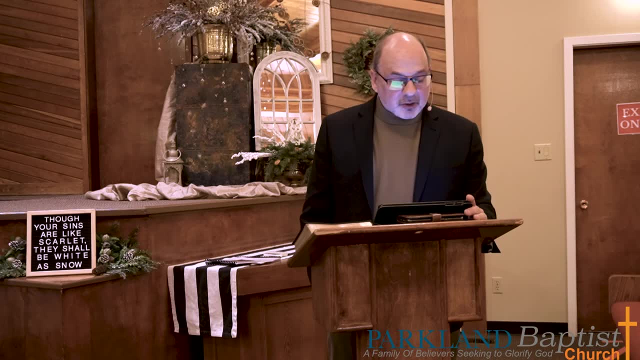 It's just to say it'll be a looser understanding of the original meaning. So the authority in a reader-centered and an eisegesis, the authority lies with the reader, not with the author. In fact, This hermeneutic is not limited to the scriptures. 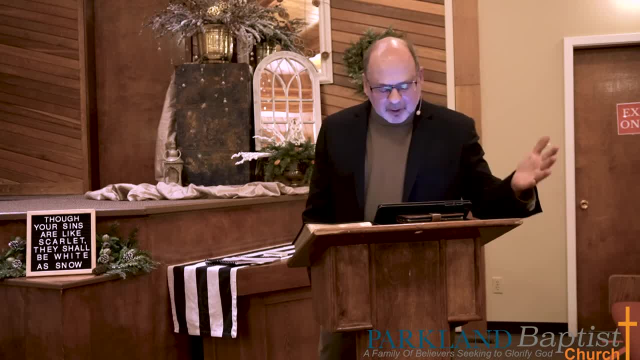 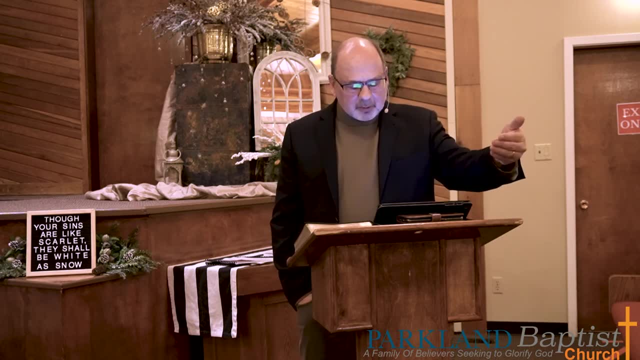 This is common in the judicial system. In fact, I remember when Amy Barrett was being, you know, voted in or whatever into the Supreme Court, She kept saying that she is an originalist. She kept saying: I interpret the Constitution as an originalist. 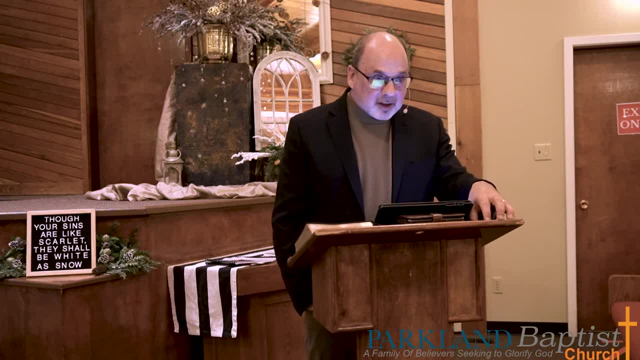 What does she mean by that? What she meant is that, whatever the original framers of the Constitution meant, that's how she interprets the law. Then there is the progressive, the progressivist, which is mostly the left, And the progressivist is. it's not what the original framers meant. 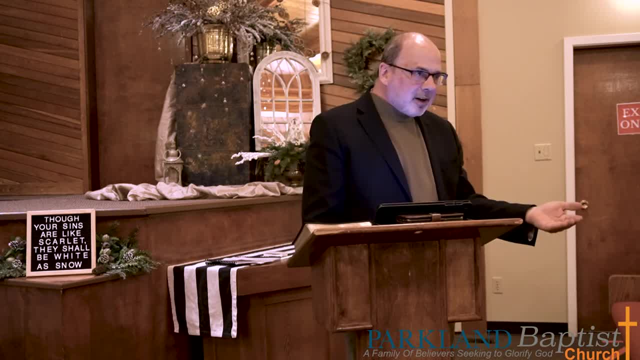 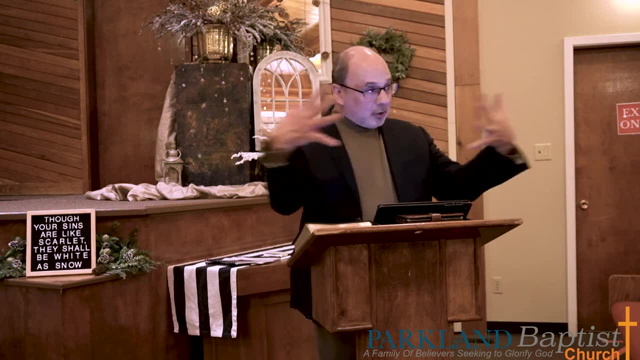 It's what it means to us today, And so when they try to read the Constitution, they read it in the context of a 21st century understanding, And this is why the two can never agree on what the Constitution means, Because the originalists are going back to the original framers. 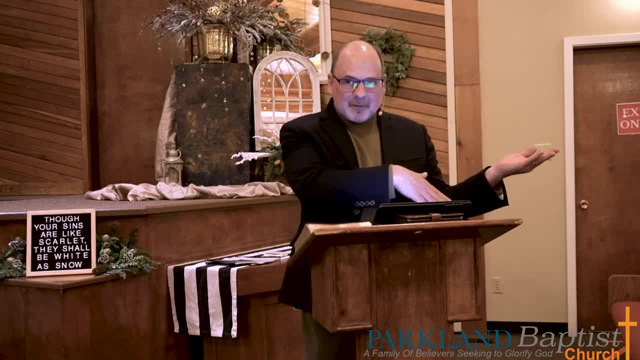 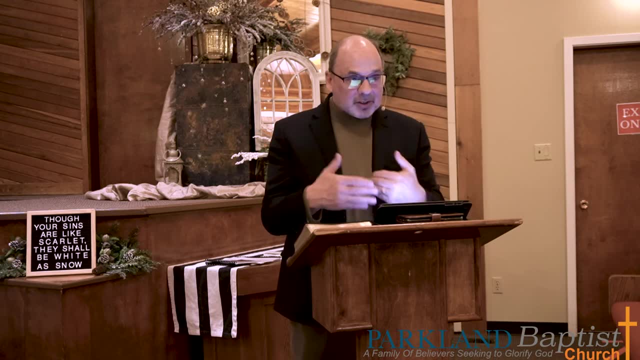 The progressives are saying: no, it means this in the 21st century. Okay, So as interpreters of Scripture, we need to be originalists, not progressivists. Originalist means that we stick to the original meaning of the text. 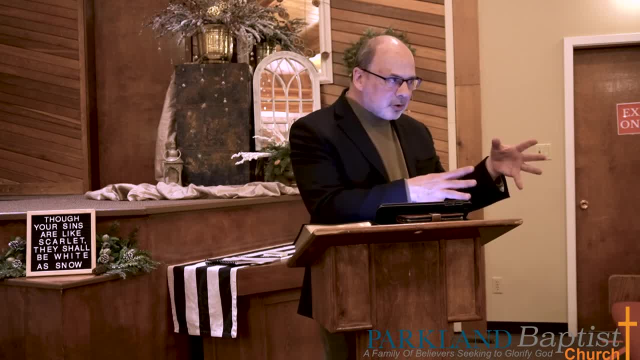 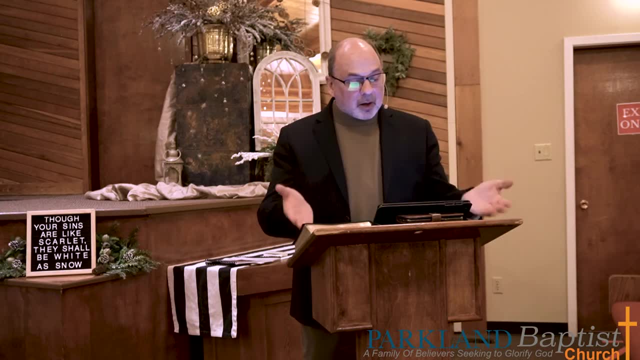 The progressivist will say no, it has a new meaning today because we live in a new age. So that's eisegesis. Now, exegesis is exo, the pulling out of the discovering, the bringing out of the original meaning of the biblical text. 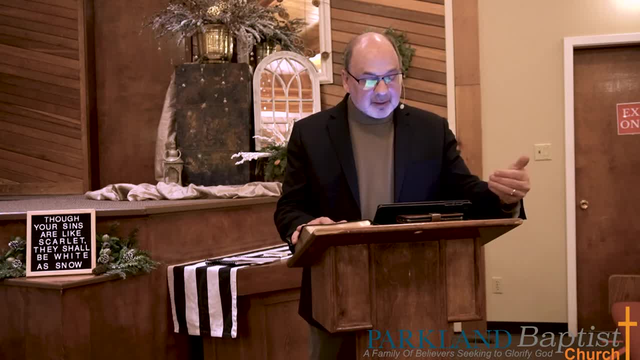 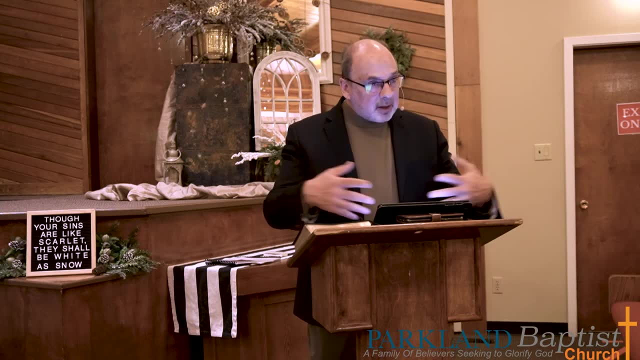 By studying the passage according to the author's intent. This is when you've got to take into consideration the history of the time that it was written, in, the culture of the time that it was written in. what kind of literature is being used? is it poetic, is it historical, narrative, is it figurative, etc. 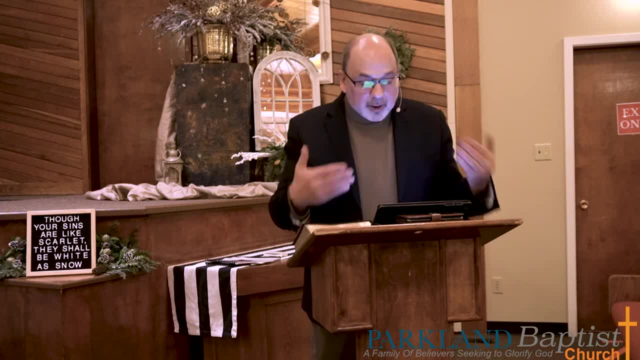 You've got to take all those things into consideration when you are trying to draw out the intended meaning of the text. Okay, So in the end the Bible was written, I believe, in such a way that its teachings are able to be understood by all people. 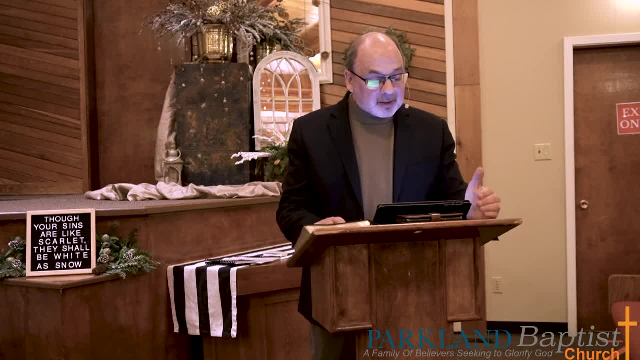 who are willing to study it in submission to the Spirit of God and who are willing to obey its teachings. I believe the distortions of scriptures come when we are unwilling to submit to certain teachings of scripture, And that's when we start to say: well you know, maybe it means this and not that. 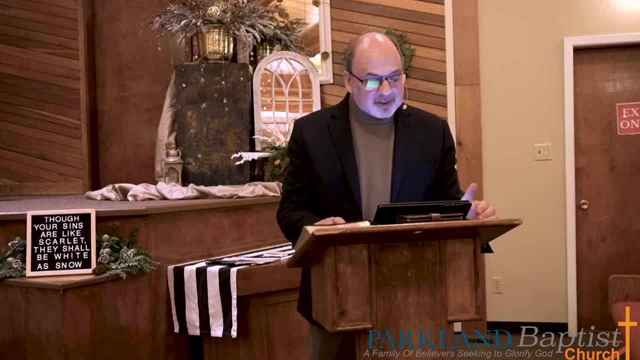 So 2 Timothy 2.15 says: be diligent to present yourself, approved by God, as a workman who does not need to be ashamed. be diligent to present yourself, approved by God, as a workman who does not need to be ashamed. be diligent to present yourself, approved by God, as a workman who does not need to be ashamed.